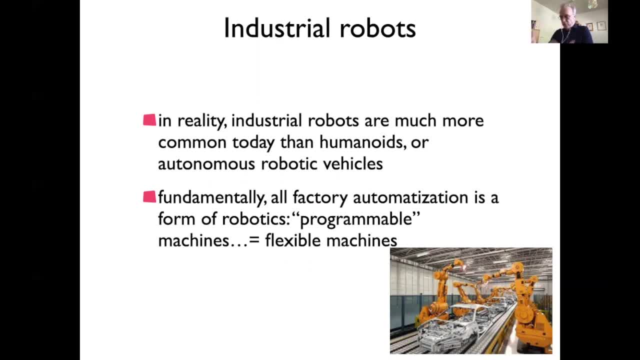 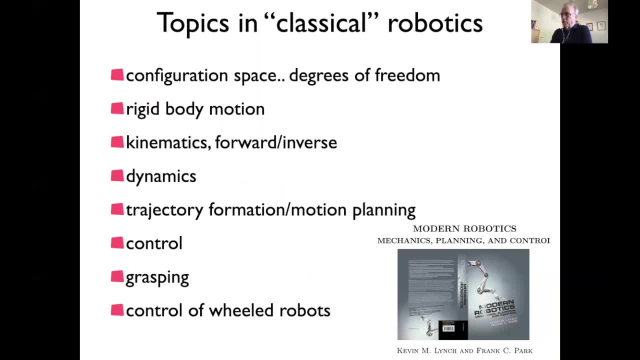 You can see that it's a little bit more complex than what you see in the real world, but it's not something that can be defined as programmable machines or machines that are flexible in what they can do And that flexibility shows up in them being programmable. 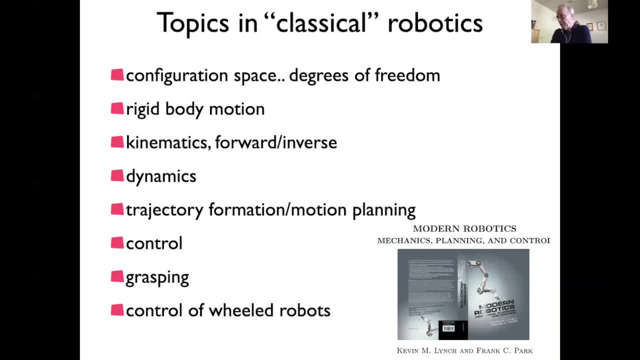 a whole continuum of actions being possible. If you look up a textbook like the one I cite here on classical robotics, you will see topics that relate to that. So it's about how to describe mechanically, it's about the kind of motions these artifacts, these manipulators make rigid body motion. 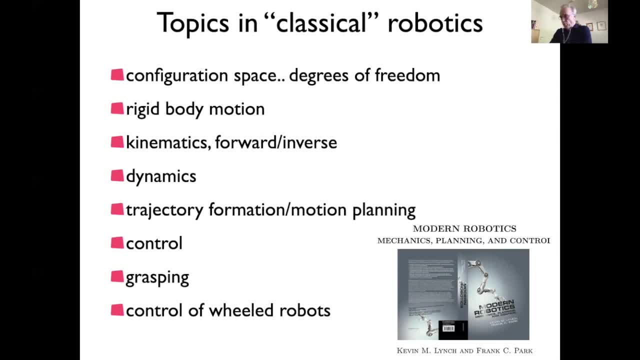 about their kinematics, forward and inverse, or computing where they will be in space, or computing what kind of joint angles to make to come to those positions, Their dynamics, physical dynamics, trajectory formation, designing the time courses of the movements and the paths, motion planning, controlling. 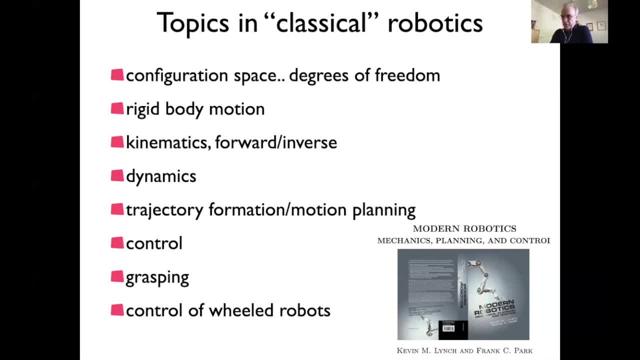 these, So making sure that they actually do follow those plans, and maybe there's something about grasping sometimes and something about controlling real robots. So the only topic among those that overlaps with artificial intelligence research is really the motion planning trajectory formation topic, And so I will not be really talking about these. 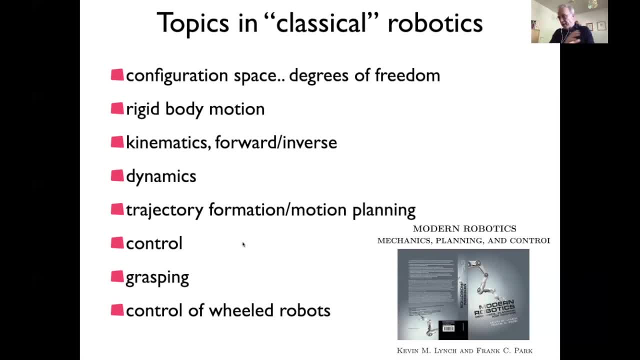 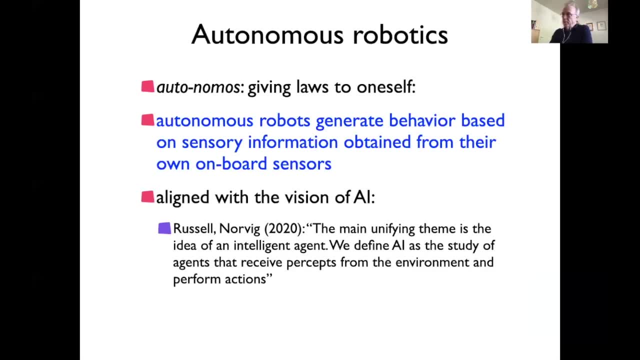 kinds of topics, just want to make sure that is actually where the bulk of classical robotics is. So in artificial intelligence we're more interested in autonomous robotics. So autonomous really means that they program themselves in some sense. right, The word comes from this Greek notion of normus: giving yourself the law, auto normus. 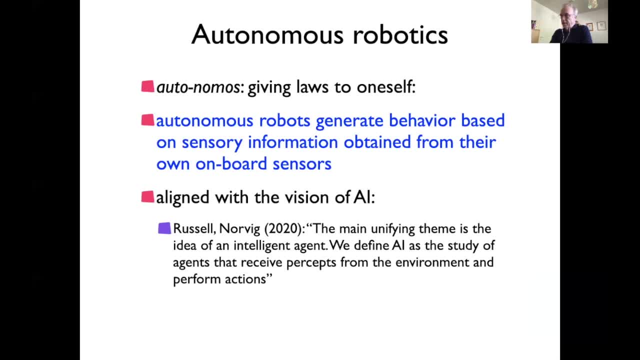 And technically we mean by that that these robots generate some form of behavior, some movement, ultimately action that's based on sensory information that they themselves have a acquired, that they are informed about what correct actions or desired actions are, based on their own perception of the environment. And so, if you remember my first lecture in this, 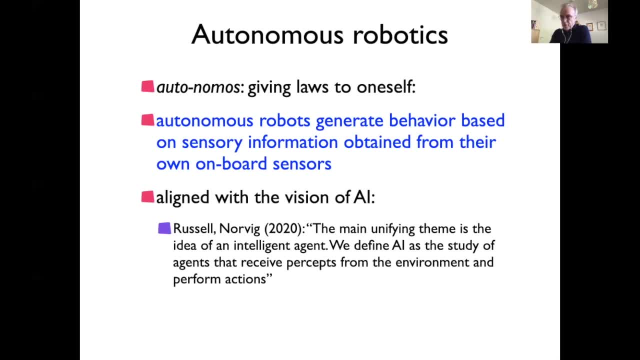 series about cognition, and then you see that that's very much aligned with the vision of artificial intelligence. I then quoted from the textbook of Russell and Norvig that the idea of an intelligent agent is a unifying theme in artificial intelligence, And they even define: 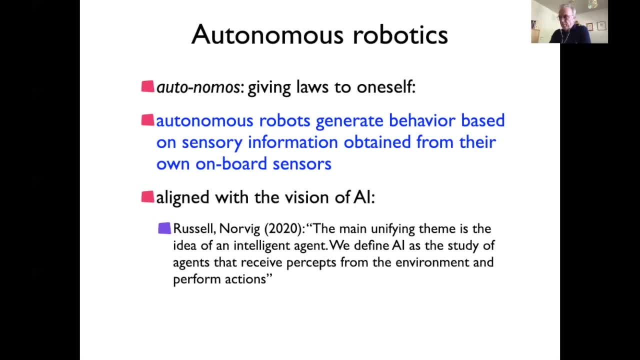 artificial intelligence as the study of agents that receive percepts from the environment and perform actions. So that's the definition essentially of a autonomous robot. It's maybe the only question is whether the agent really has to be physically able to act, or would it be acting? 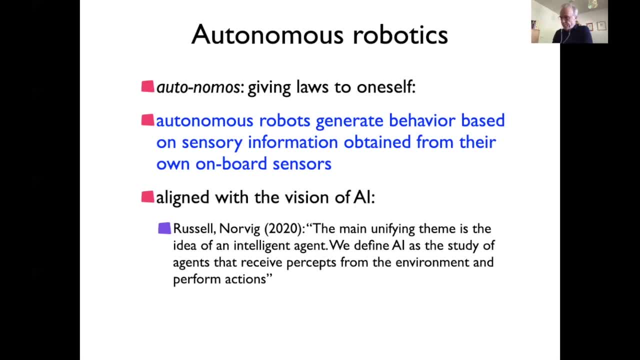 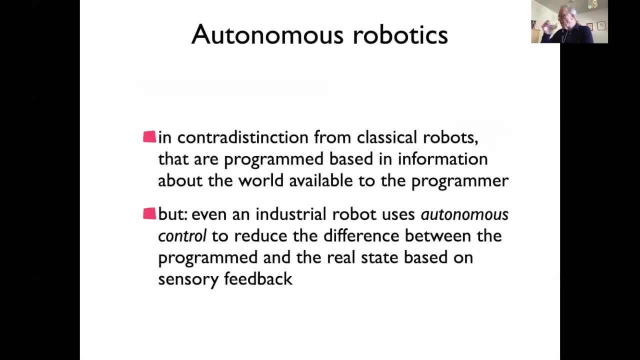 just informationally, for instance by talking to someone or giving some response on a computer screen. So so this notion of be struck, organizing one's behavior based on sensory information that is acquired by the robot, is, of course, in contradiction with the classical robots that are programmed and they're programmed. 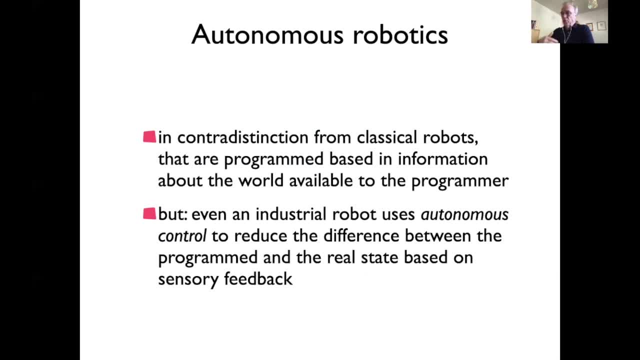 based on information about the world that is available to the programmer, not to the robot itself, to the robot system, Even though So a industrial robot will also have something that's called autonomous control, which is essentially to make sure that it really physically realizes the planned motion, the programmed motion, and it does that based on sensory feedback from shaft encoders, kind of sensors about its speed and position, and it will control by reducing the deviation between the plan and the real state. 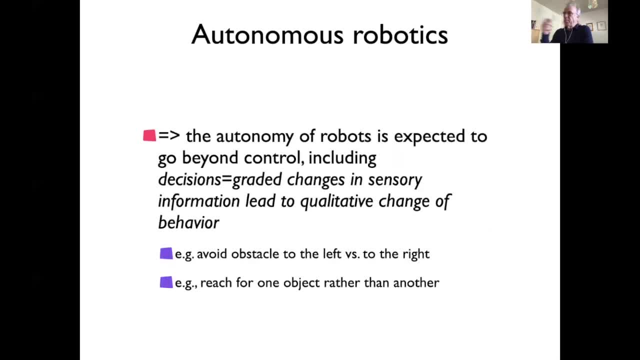 So that form of autonomous control is not what we mean by autonomous robotics. In autonomous robotics, we expect something more, something not as simple as that as just achieving a set value, And one way to talk about that is to say: we are looking at systems- autonomous control systems- that also make decisions. 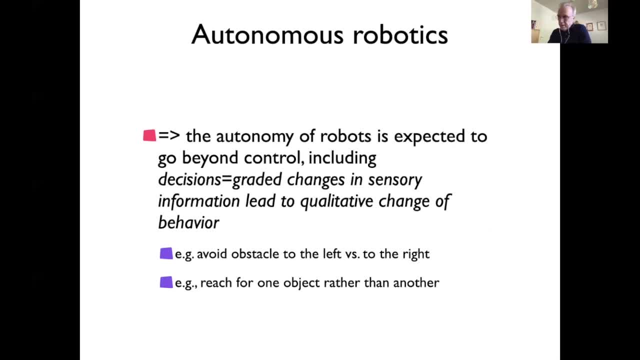 So decisions ultimately, in the simplest form, mean that some greater change in sensory information will lead to quality difference. So that's a very simple example. if you automatically avoid an obstacle, there will be a critical point when you will decide autonomously if you avoid it around the left or around the right. 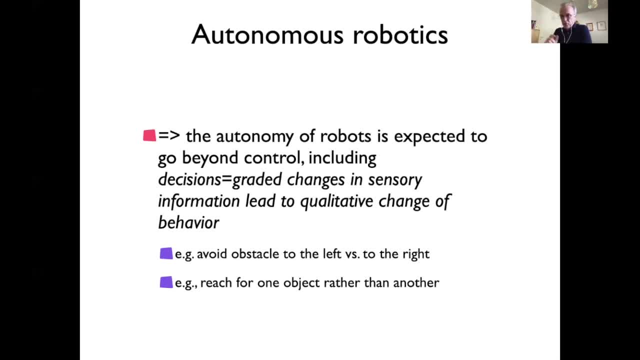 A small difference in sensory information will lead to that macroscopic difference. Or, you know, you might want to orient your action to one object rather than another, depending maybe on how closely they match the description. there will be some critical point when you switch your preference to another object. 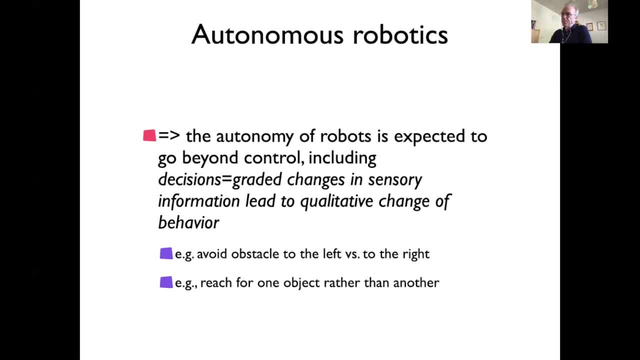 Or you might want to orient your action to one object rather than another, depending maybe on how closely they match the description. there will be some critical point when you switch your preference to another object. There's many more complex ways to talk about that, And those are essentially the ways to talk about cognition, as I did in my first lecture. 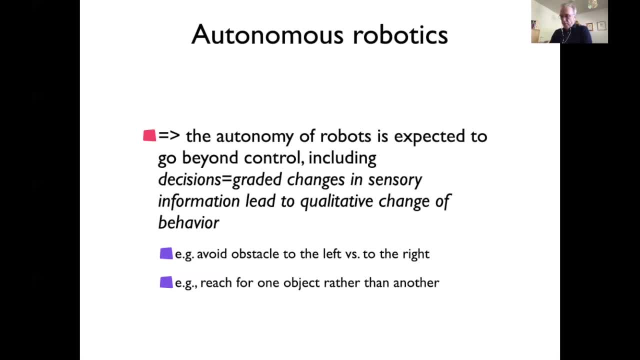 So cognition as revealing a more indirect link. systems become more cognitive, the more indirect the link between their sensing and their acting, and the decision would be sort of the first milestone in becoming conscious and aware. So this gives us an idea of what the act is actually like. 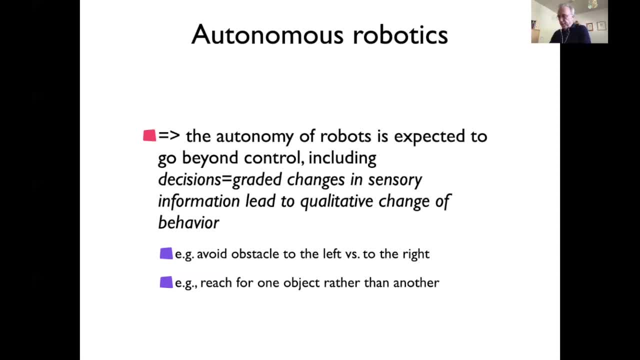 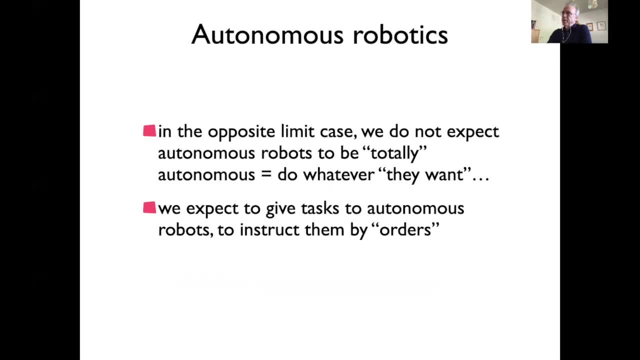 So cognition is to detect and empathize dzięki negamima indirect, where the input doesn't uniquely determine the output, Memory would be the one, and sequences and so on. So clearly that's the you know, to demarcate autonomous robotics from. 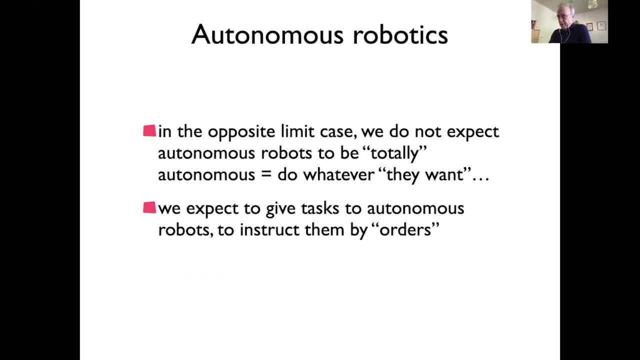 control. In the opposite limit case, we also actually don't really think of autonomous robots as being totally free to do whatever they want, in a way, right And concretely, that means that we typically expect these robots to take commands, you know, to do tasks that we instruct them about. 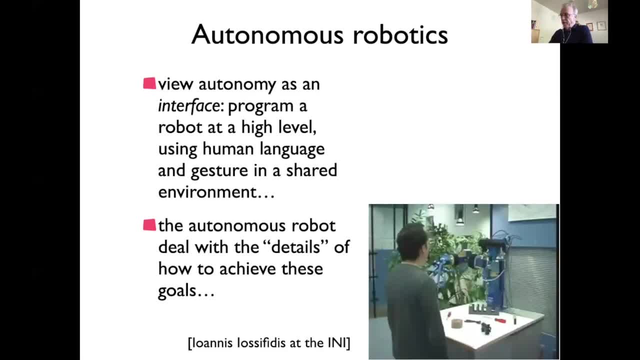 by giving them some kind of orders, And in fact here's a demonstration of someone at the institute did this work a long time ago, where he interacts with a robot giving verbal commands, pointing at objects, and the robot will do things then, And so that is actually a very 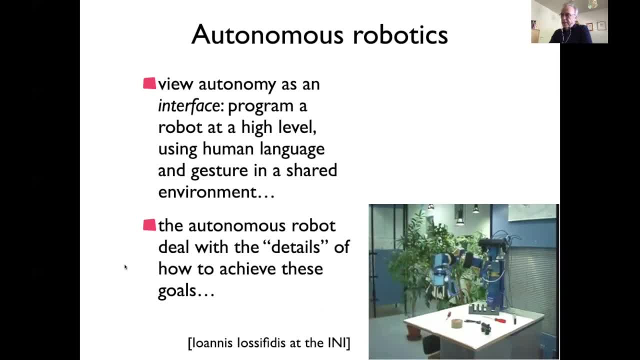 plausible use case In which the autonomy is essentially setting up an interface. So you still program the robot, but you program it now at a high level by talking to the robot with human language, maybe with gesture, both immersed in a shared environment, an assistant. 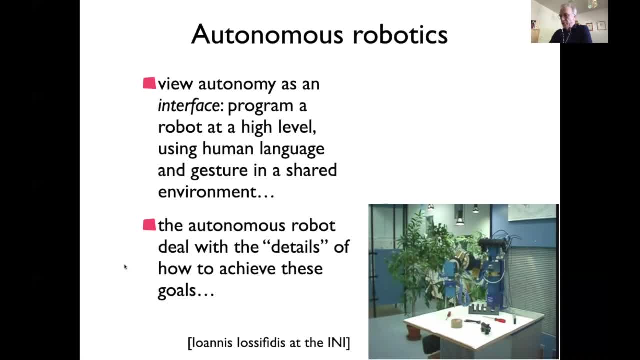 robot, And autonomy then consists of the robot filling in the details. When you program the robot in a conventional sense, you would have to give it all the details. you know where exactly the object is, the coordinates and which joint configuration it's going to be. 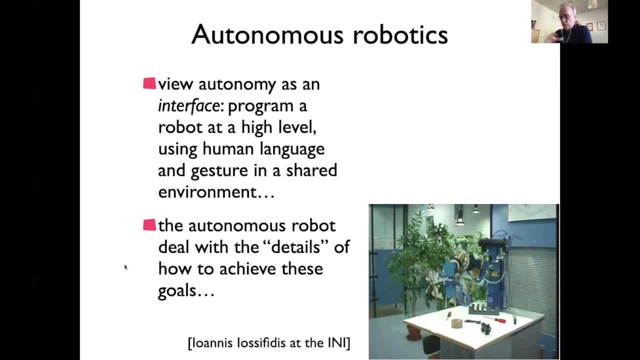 You know which joint configuration exactly to use, with which speed and so on, which grasp, And being able to just set the goal as this macroscopic level like get me this object, then the generation of the detailed solution to that would be the autonomous part. 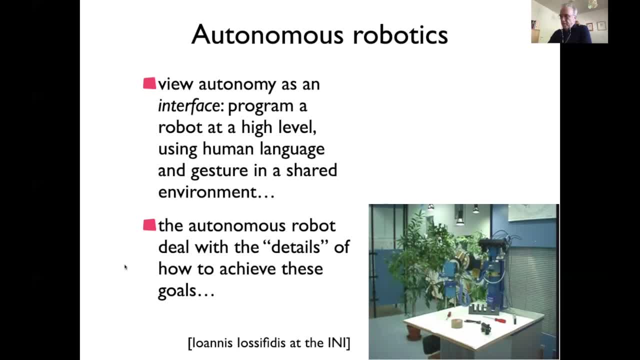 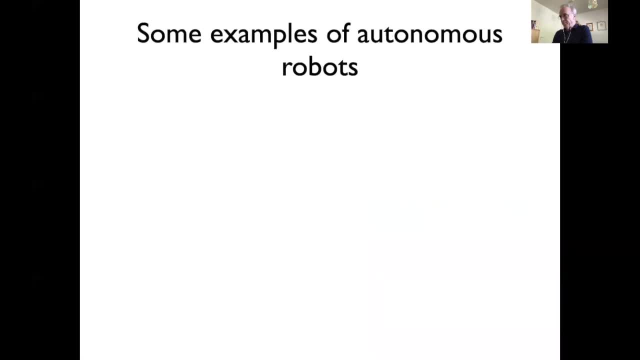 So in that sense, autonomous robots could be viewed as robots that provide this kind of high level communication interface, And that's an idea very common in assistance robotics. I wanted to give you a survey over some typical autonomous robots, took some images- not all of them are very new- just to make a landscape, And that will prepare one point. I'm 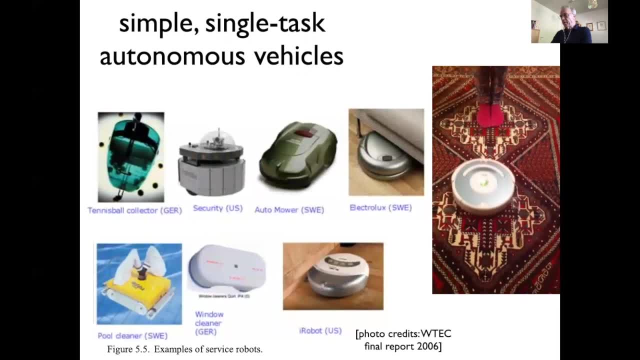 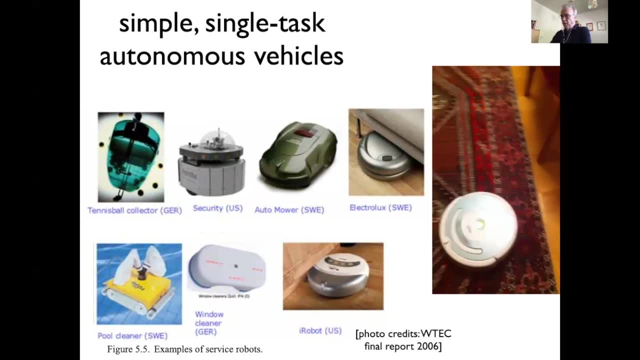 going to make next. So here one thing that is commercially available. I actually own this little vacuum cleaner. you know you can buy those for not not very much money. now there's a whole bunch of single task vehicles, And this is not the latest. 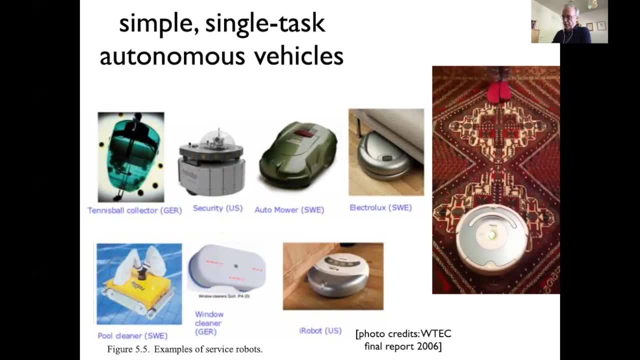 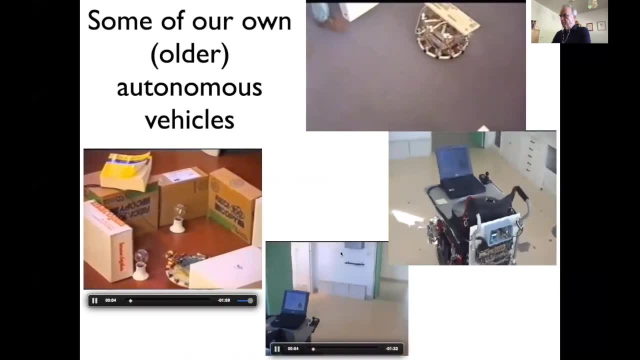 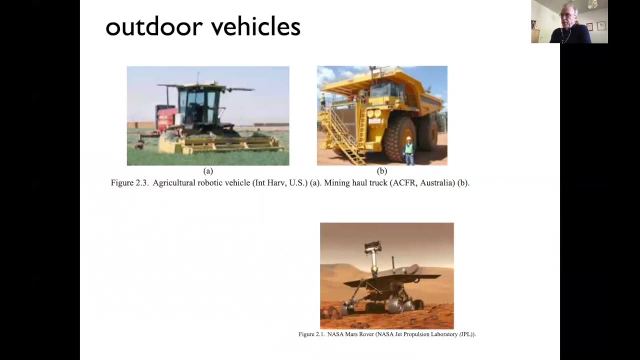 that do these tasks autonomously with their own sensors and so on. so that is, uh, well established. uh, we actually built some of those back then i'll show you one example of also the sort of research tool. um, then you, you can have vehicles of other kinds, you know, outdoors also special tasks. 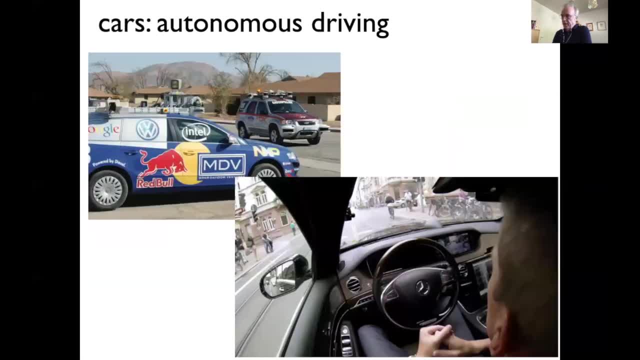 uh, the more special tasks, the more successful. these kind of things, uh, and of course there's kind of striving and turns, driving, as you will know from the media and so on- has made enormous progress, is becoming close to being feasible in in daily life and it is a form of robotics. 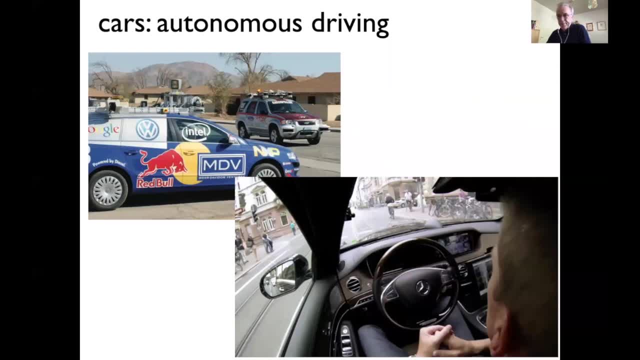 it's not always perceived to be that, but by its very nature it is autonomous robotics and i'll refer to it a little bit. i will- most of my survey will not really, uh, focus on on that, and you'll see why in a moment, but i will be referring to that a couple of times. 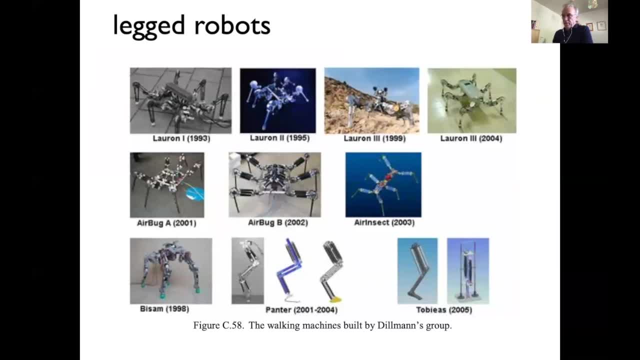 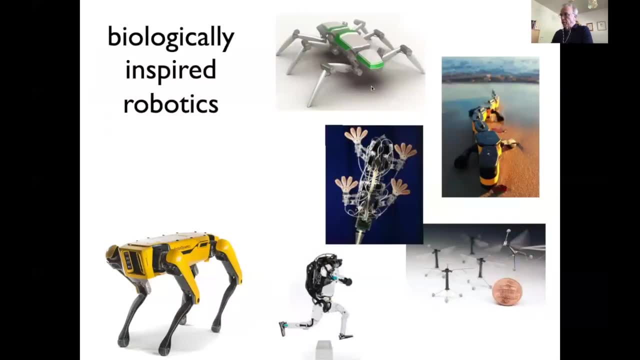 another form of vehicle are legged robots. which vehicles? also? because they move around the world and carrying the sensors along. they are very often inspired by biological analogies, you know, insect-like robots or sort of salamander like robots, uh, dog like robots. this actually human. 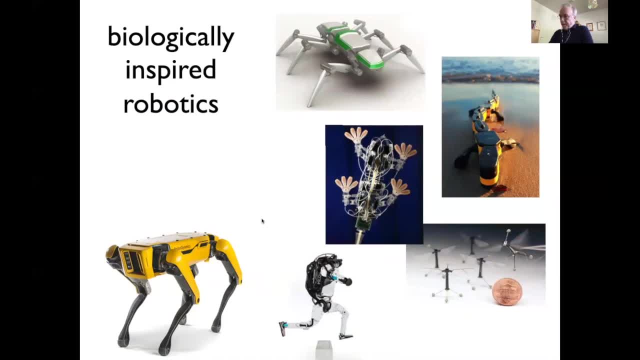 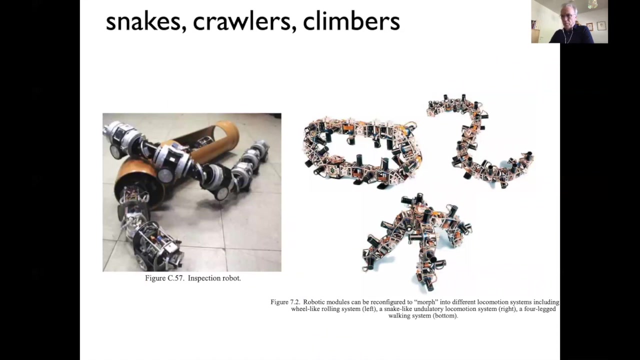 like robot, so it's an animal, um, and they're, they're, provide a form of locomotion. so there are vehicles in that sense, uh, and they have this advantage of being more flexible with respect to the surface that they walk on. and biological systems, as you know, have not developed wheels. um, also somewhat biologically analogous, are some special purpose. 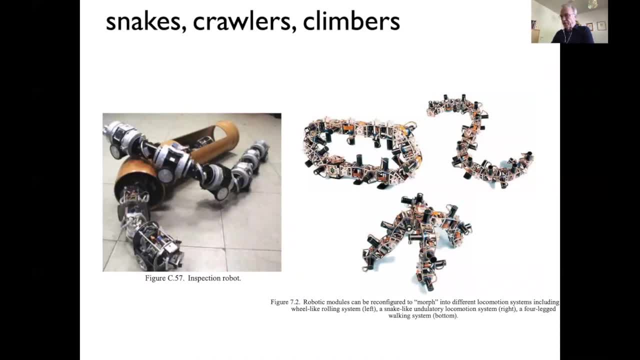 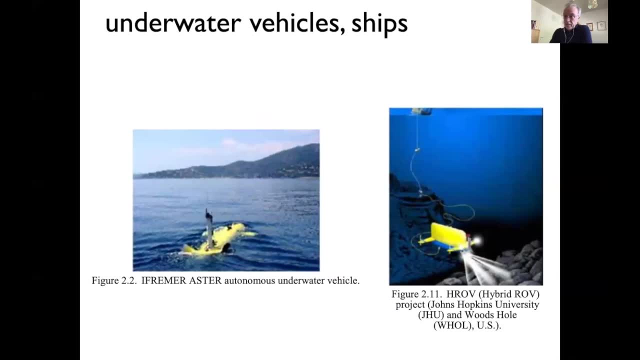 kind of robots that crawl or can climb or snake like and so on for special purposes. and then underwater vehicles are commonly looked at as autonomous systems, so inspired by fish, if you wish it's. it's easy as a medium because it's a homogeneous. it's mostly a communication problem. 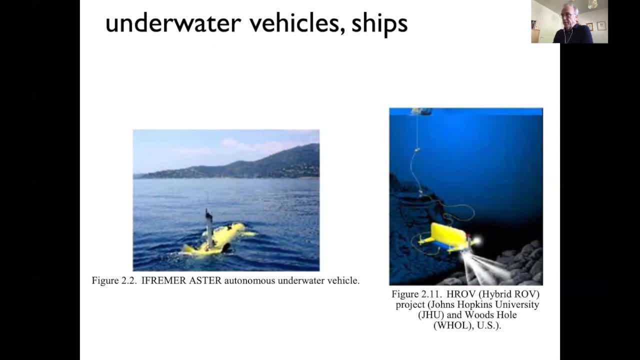 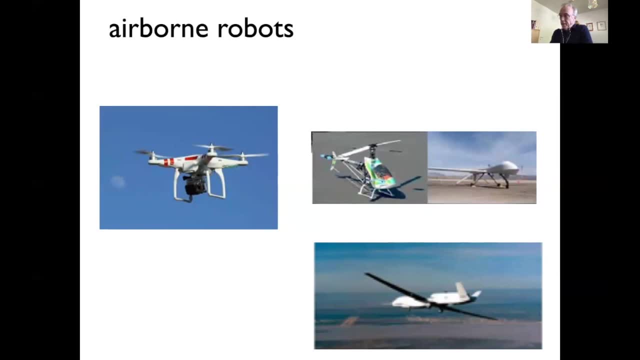 underwater, and but it's a legitimate form of autonomous robotics. and then, of course, flying robots, uh, drones, as you know, are very common and again, they are, uh the autonomous. very easy, in fact, commercial aeronauts are an autopilot, but very often, in that sense they are autonomous, then, 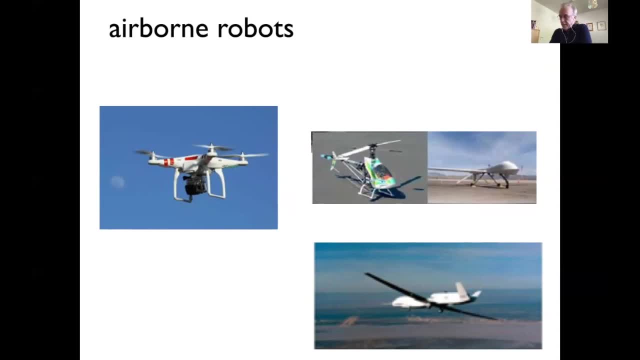 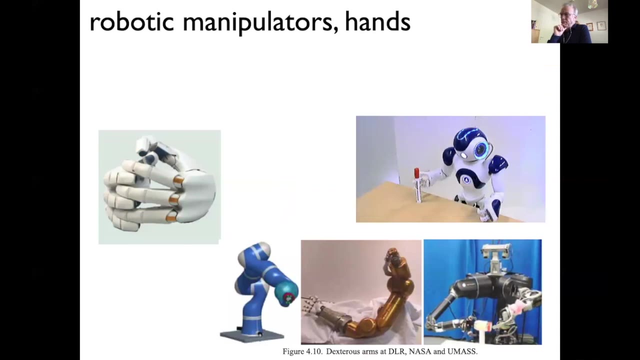 the decision making, though, is made remotely, and that's one of the frontiers of making systems, uh, autonomous in this wider sense of, uh, you know, going beyond control. now, robotic manipulators, or arms or hands, are a different story, so they are, in some sense, analogous to. 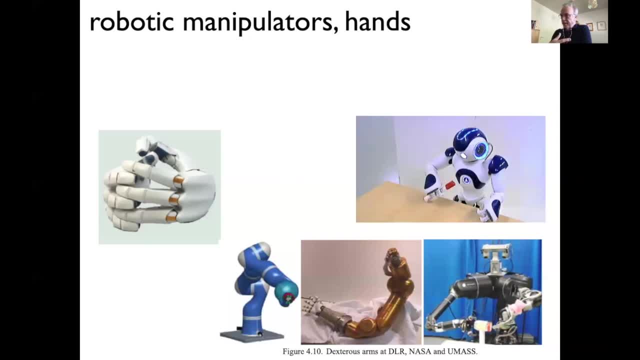 industrial robots. but now you're thinking about a robot that is autonomous, for instance, that would perceive an object and then orient its action to an object, grasp it and handle it and so on, and that autonomous part is actually very difficult. so autonomous manipulation is one of the frontiers, it's not. 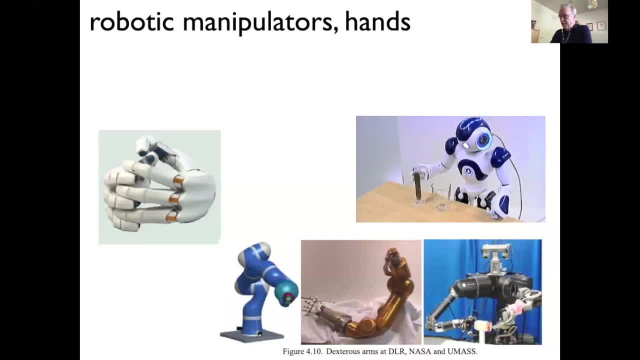 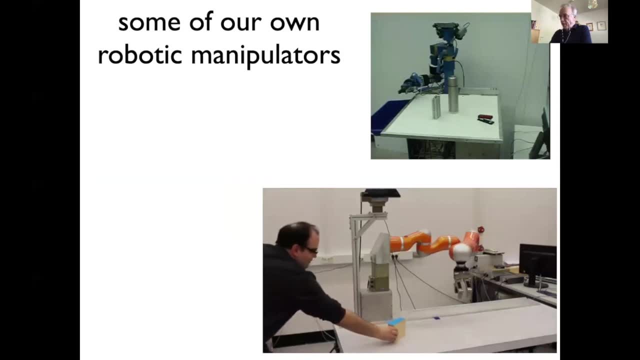 very much successful work in that domain. i'll be talking about some of the difficulties and then you can. yeah, actually we in our research also look at things like that. so here at the bottom, that's one of our systems that is supposed to grasp objects. uh, based on its own vision, you. 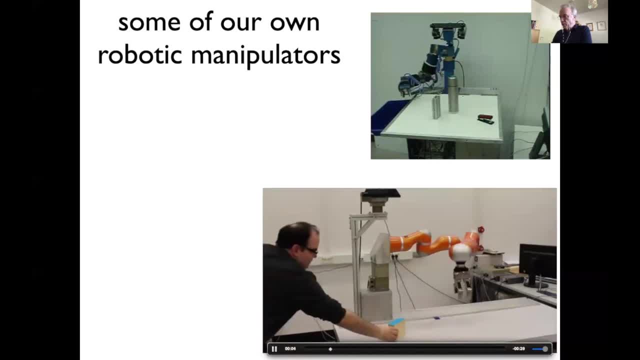 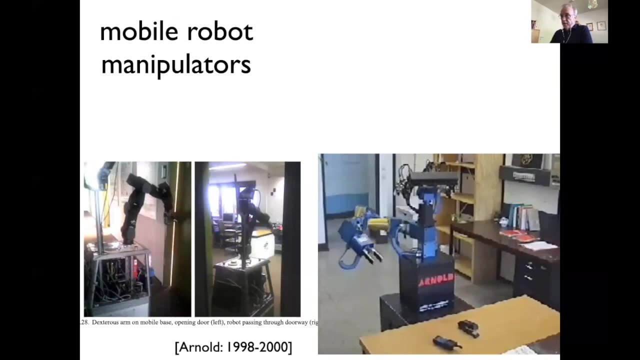 just saw that the object was moved around just as it was approaching, and that's one of the features that is able to update its plan. now, here another case: update its plan as it is being, uh, as it is acting, and then you can put the arms on a vehicle and then you have a mobile robot manipulator. 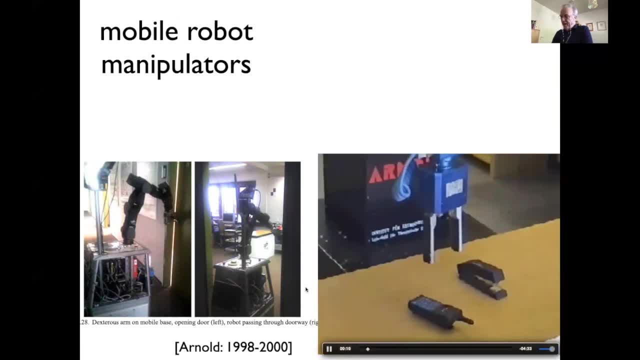 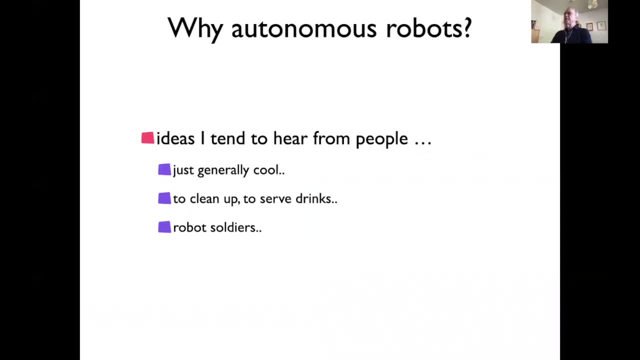 and that is also a human interface here. uh, that, you know, combines all these problems. so get the picture, perhaps, what overall that field is. so why? why do we do this? why are we interested in that? when you- i ask people occasionally, including my son, about that- and here are three responses i get- 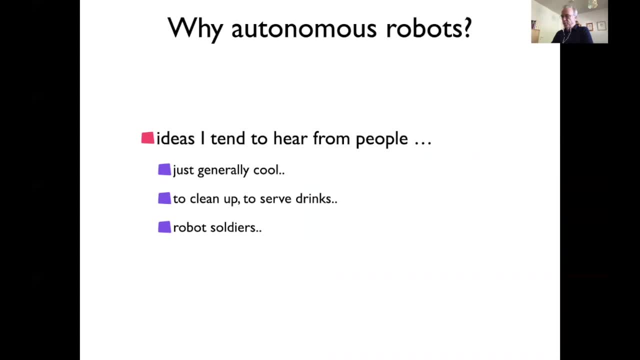 which actually do match or line up with some typical use cases. so they are cool, fun systems to have, like all the movies are about that. uh, they could serve me, like serve drinks, or clean up the kitchen, or they could be soldiers, you know, without humans then having to do their job. and 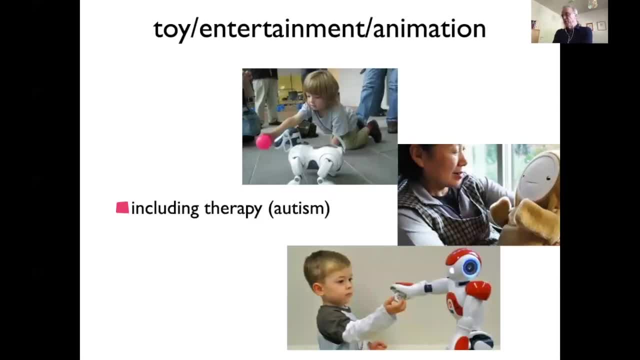 those are three use cases actually. uh, useless robots that are toys or for animation or entertainment are actually the first real commercial uses. there's some robots that are sold for that purpose. there are some famous case that some autistic children tend to react better to robots than to humans in some sense, but it's a. 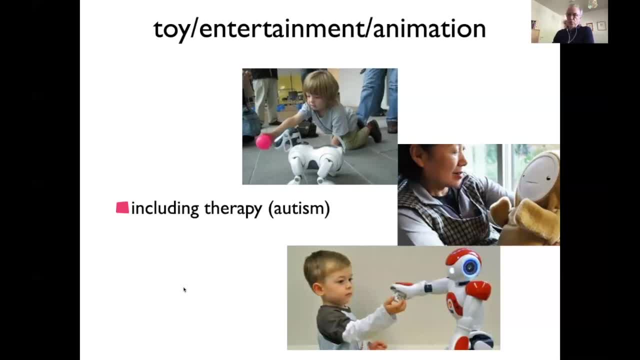 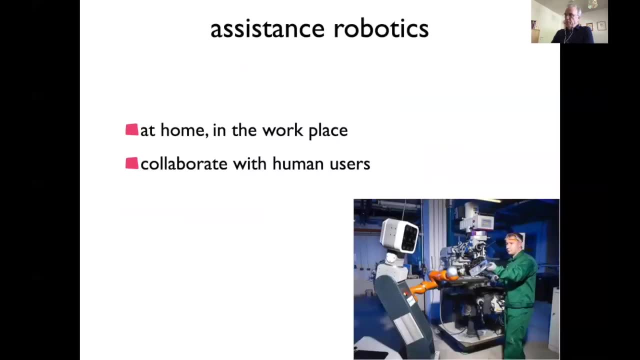 very niche application so so that's sort of a purpose-free way of using robots. it's very popular in some regions in japan in particular, and the other big vision that's very popular in europe is the vision of assistance robots, so robots that will, at the home or in the workplace, collaborate. 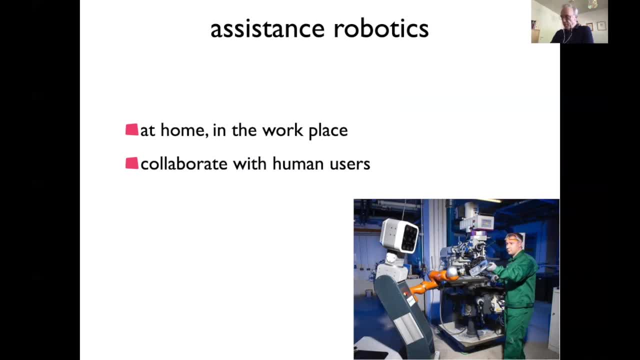 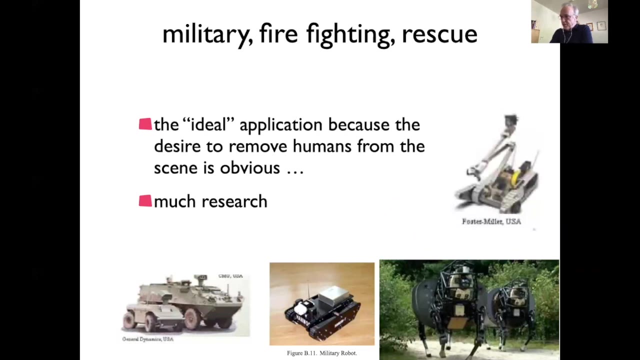 with humans. it's very demanding, so a lot of problems need to be solved to do it, and i'll talk about some of those problems later. uh, it's not a reality. it's a research enterprise, um, and the military robotics does exist in a big field. that is not so. 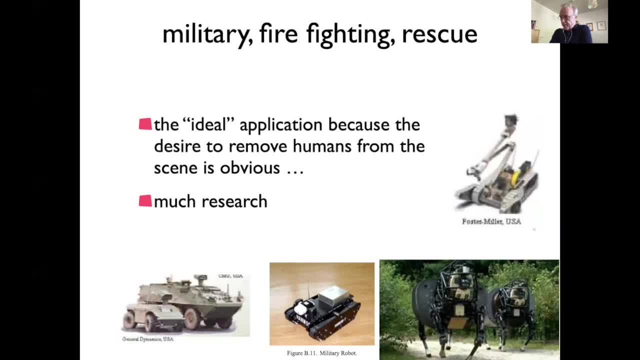 well known, because most of the work is confidential or not done in universities, for instance. it's ideal as a technical application, in that the need to remove humans from the scene is obvious and the environment is difficult, as we call that natural, hard to model. could change. so it's. it's a could be hostile, um, various kind of threats you have to detect, and so on. so it's i'd. 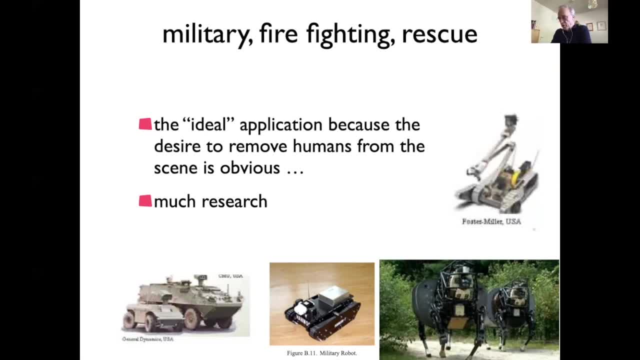 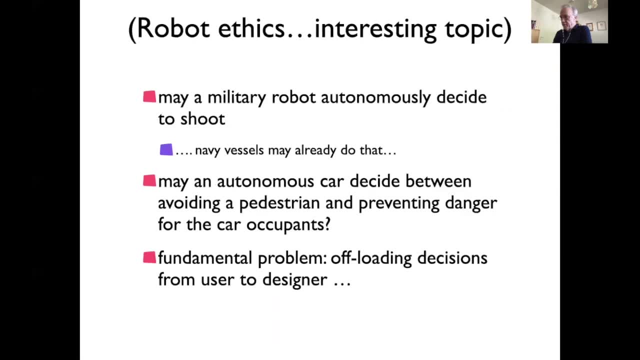 deal for for this kind of research, and there is much research on that in europe- it's not not as much as in the us and probably in russia and china. as a side aspect, this is often the opportunity for people to think about robot ethics, which shows up in robots that act. 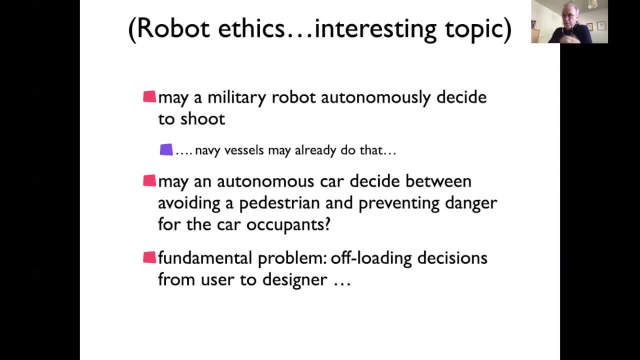 autonomously only right, because then you have decisions being taken and are these decisions subject to some kind of ethics? so in the military case people ask: you know, can you, you know? is it admissible to have a robot decide autonomously whether it opens fire or not? there are actually already, maybe, vessels that are conventional, you know? but 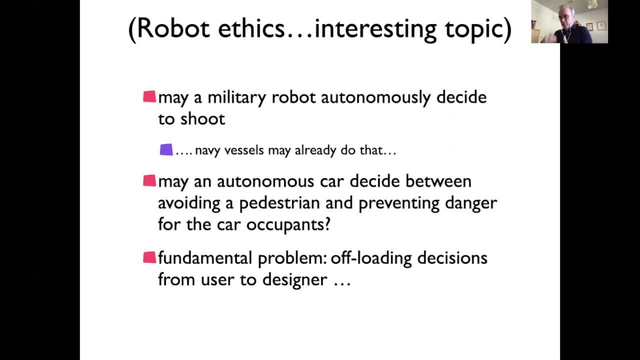 they are in some sense robotic, autonomous when they are in a certain mode of battle configuration where there's a human who can override commands, but they a priori decide autonomously, for instance, to shoot an anti-aircraft missile that's been around for quite for decades. 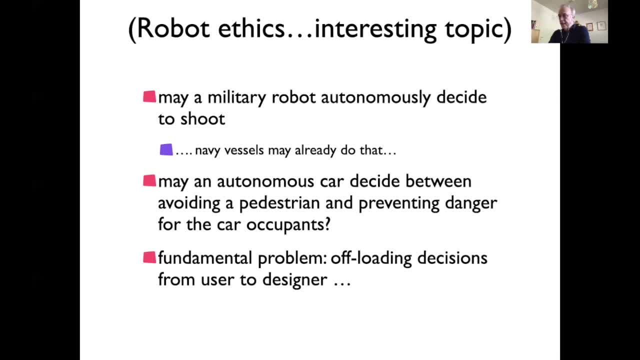 so these issues are real. uh, as we look at autonomous driving, issues like that come up. for instance, if you detect a possible collision of the pedestrian, on the other hand that an evasive maneuver might lead to a crash, you know which which are going to who prefer the? 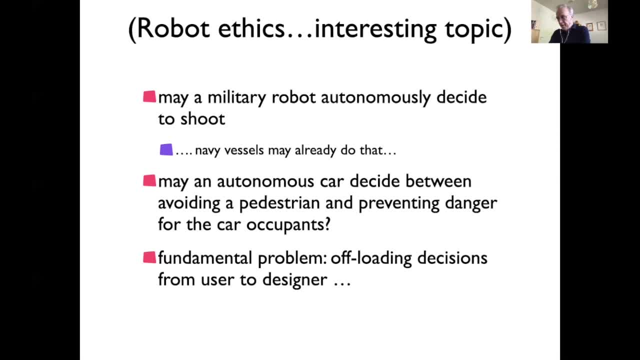 owner who bought the car? maybe it's your customer or do you have some, you know, value hierarchy built in? so there's a lot of debate about that and there's some interesting work by philosophers- or i'm not sure why this is this one, or you know. there's some interesting work by philosophers. what are you doing to measure that? and i think that's also interesting. and one of the things that you mentioned is: let's look at the 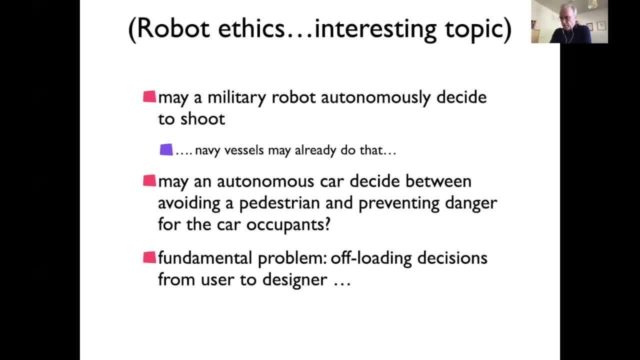 philosophers, for instance, but work like that. It's ultimately, it's a question of offloading decisions from the user to, ultimately, to the designer. You know, the robot is autonomous, but it does that according to it makes the decisions according to what the designer. 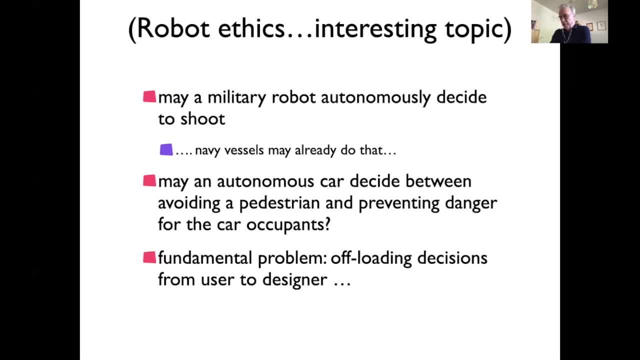 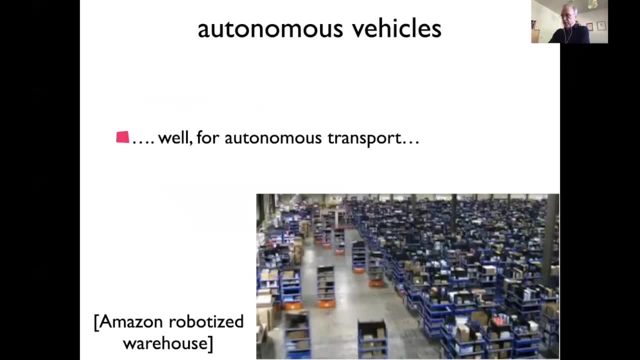 provided as an algorithm for making those decisions, And so there's interesting debates about that. I'm not gonna go deeper into that, but just pointed that. And then there are vehicles, of course, which didn't really follow those three purposes. Vehicles are for well, for driving right. 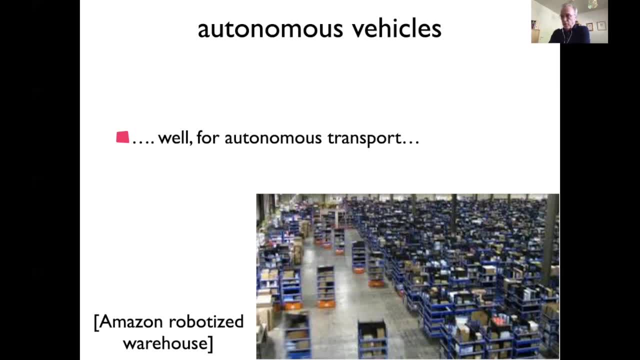 For autonomous transport, And that's a very obvious service they provide, so that one doesn't even think twice about whether that's useful. So the use case for autonomous vehicles is actually the best, And that's also one reason why they are very advanced. 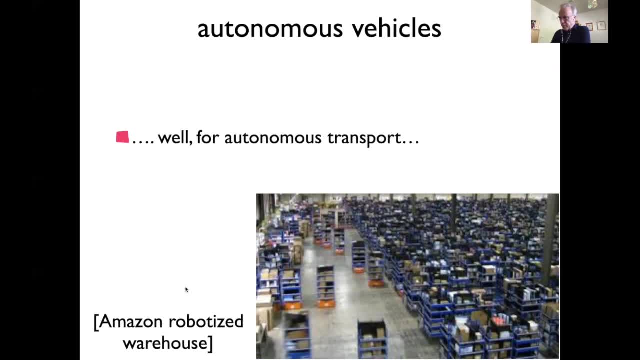 This is an example from Amazon. who has these little vehicles, these little red things under the shelves? Those are robots. They're only minimally autonomous because they will detect obstacles and then just stop if there's an obstacle, and then they'll stop And then send to base the command if there's a problem. 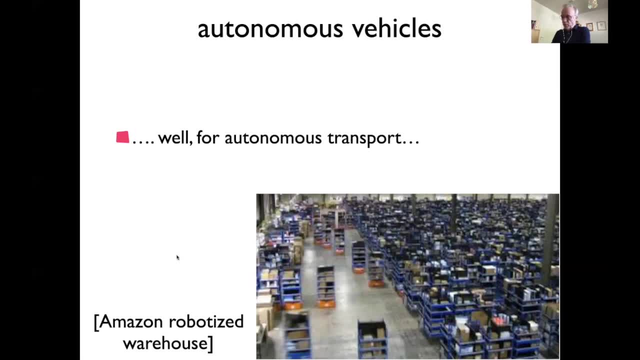 Other than that, the plan of how they move in the warehouse. that's all centrally controlled, So based on central information that's not available to the robot itself, But still it's sort of a minimal form of that. That's a very much expanding area. 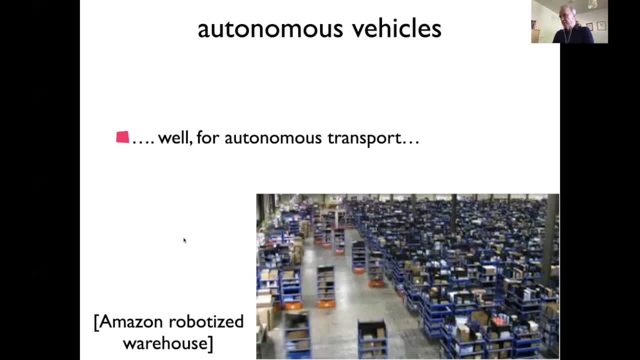 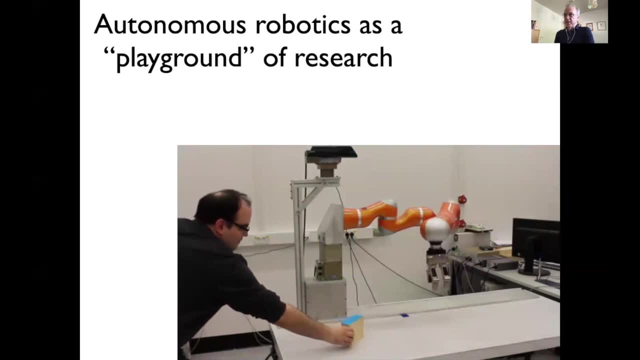 But then, of course, autonomous driving of cars on roads- that's the other big use case. That's an obvious reason why one does that. Now, the actual reason why a lot of us are doing autonomous robotics is really that it is an ideal playground. 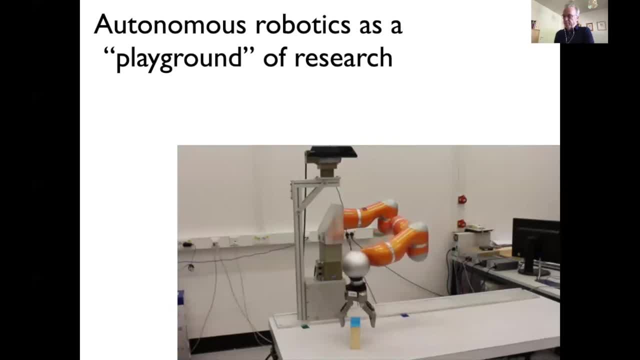 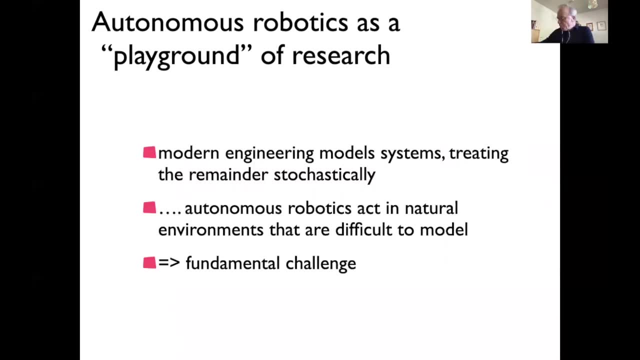 for research And I want to substantiate that interpretation a little bit. So one idea in autonomous robotics is that it is a challenge to the basic paradigm of modern engineering Could say, roughly speaking- I'm not talking just last 50 years- 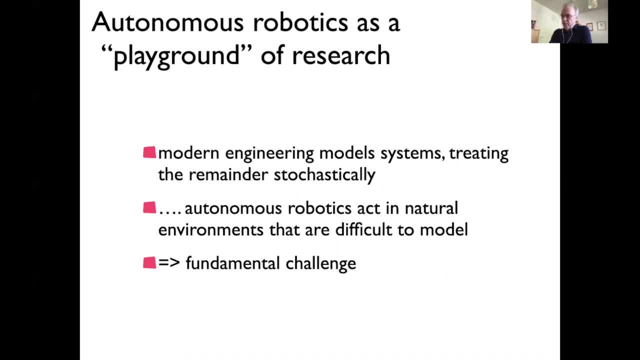 Engineering really is based on modeling systems, having very good approaches, how to model Objects, the plant itself that you control and so on, With everything that is not modeled and being treated as stochastic. So you've modeled every deterministic aspect And we have very good theory for that. 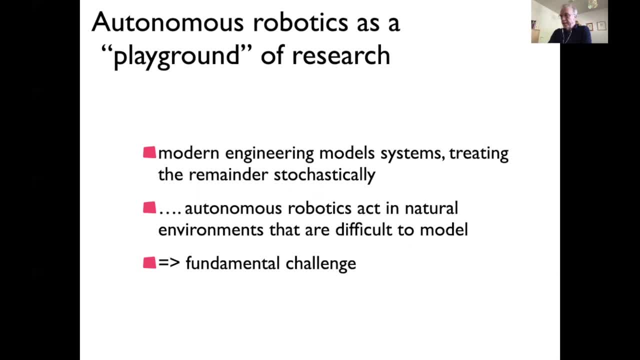 including some exact theories, And autonomous robots act in environments we call them natural environments, even though they can be factory and so on, And that really just means they're difficult to model, And so, you'll see, that's fundamentally pushing the envelope of this classical paradigm. 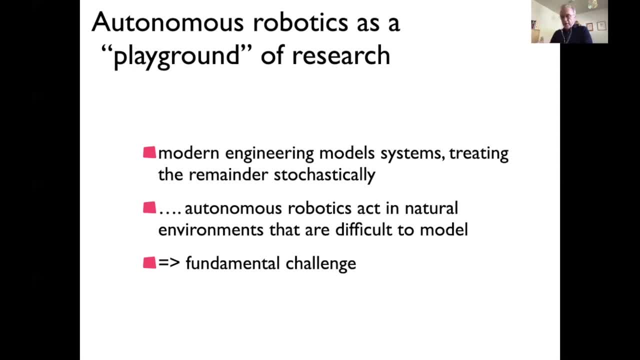 And some people react to that by saying we have to try harder to model even that. That's, for instance, done in probabilistic approaches. And others argue- and I'll see that in a while- that maybe one can achieve some things. 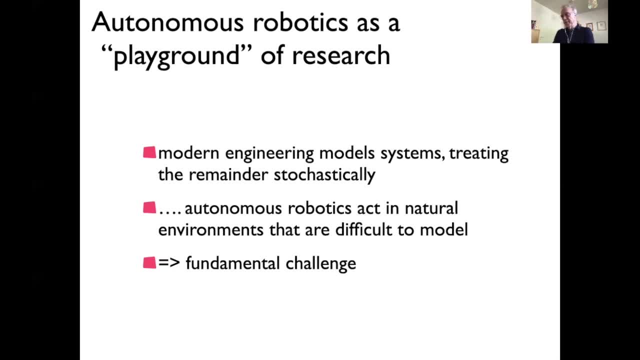 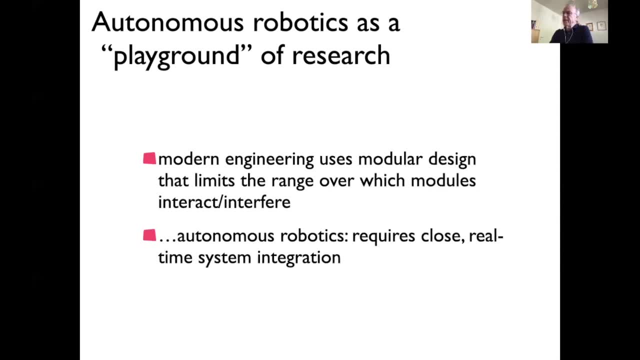 without modeling everything. So that's a fundamental challenge that robots enable you to work on. Another related aspect is that modern engineering is very much based on modeling- Modular design. So modular design means that you build components, modules which interact with other modules. 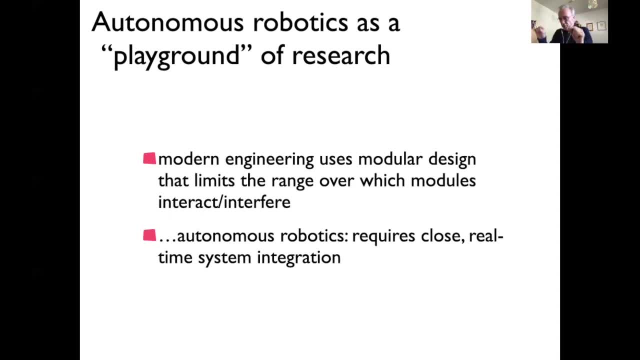 in some well-defined way, in a limited way, And that means that you can localize problems. You don't have to redesign your subsystem whenever something else in the system changes or is updated or things like that, And autonomous robots tend to require a lot. 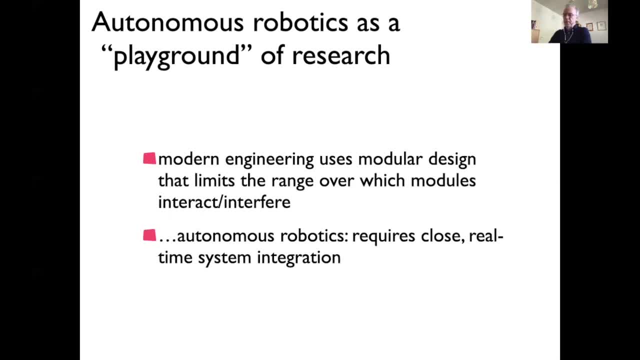 of close kind of integration- I'll mention an example like that in a moment- And therefore they challenge this. So system integration is very important and they challenge this modular view, even though modular design is still a goal in most of autonomous robotics. 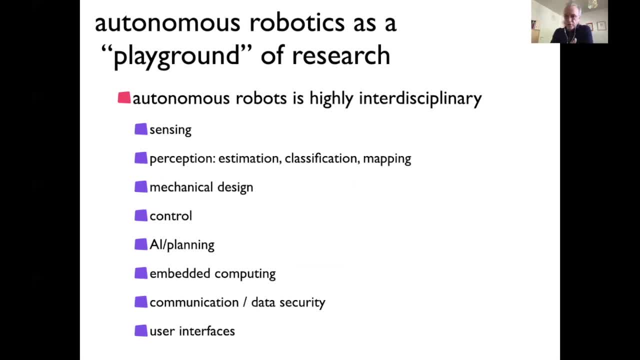 In fact, autonomous robotics is a very interdisciplinary field within engineering. I've listed here some of the necessary components that you'll have to deal with, And I have actually only listed here things that are related in a wide sense to AI kinds of problems. 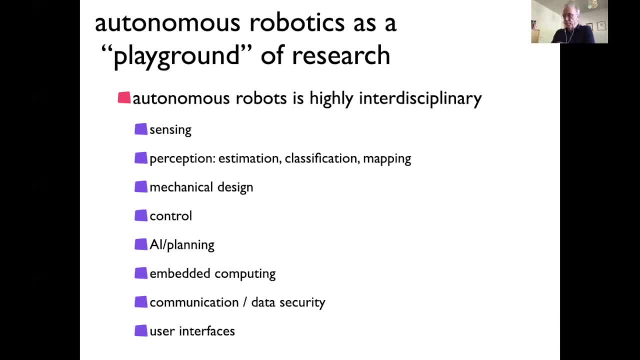 sensing perception, which is really making use of sensory information to estimate something about the world, to classify objects, to map the world. The mechanical design which often is thought of being part of the solution, which can be intelligent, adapted to the task. 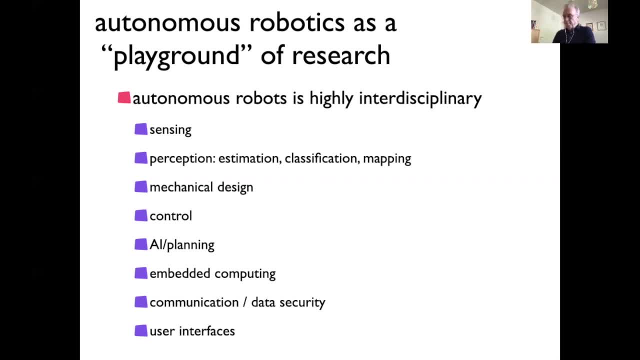 Control, of course, AI algorithm of planning, embedded computing doing all those things on a platform with limited resources, Communication among processes and with the user data security issues there, User interfaces, human factor issues and so on. So there's a lot of different disciplines. 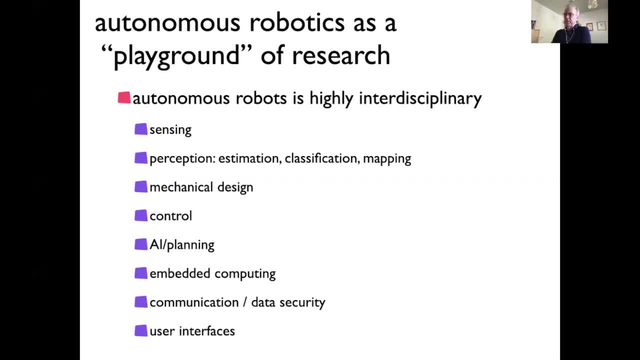 that are all integrated on a single platform. And what I did mention is some of the things like energetic autonomy. There's very interesting stuff about that. If you have outdoors, you have all the resistance to temperature and weather and a lot of other things. 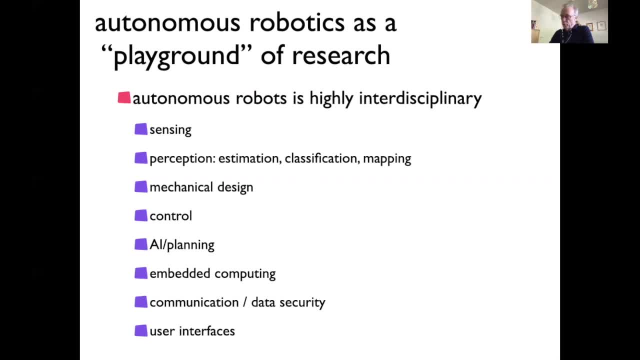 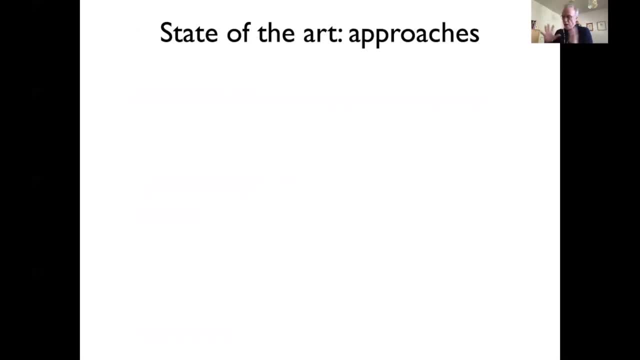 that's very interesting as a research field. So that's a little bit why we do that As a drive-in, and I'll be, of course, focusing largely now on the research perspective. I'm not going to give you a state of the art. 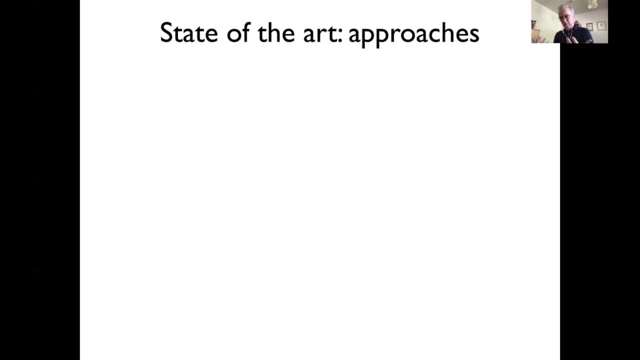 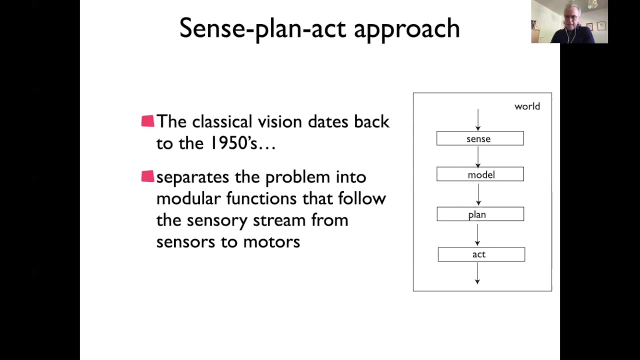 in terms of benchmarks and performance, but I just want to give you a little bit of a feeling of kinds of approaches. Really just be talking about two approaches that are commonly used in designing autonomous robots. So the classical vision dates back to the beginnings of autonomous robotics as a field. 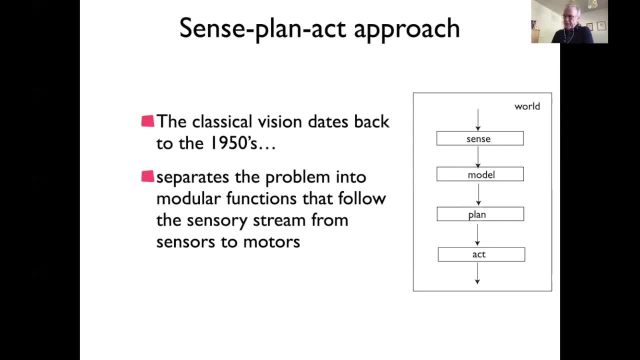 as a serious field, Not in some place, But it's a field. It's a field, It's a playground. It started in the 50s. Shakey was maybe the first serious effort, And these systems had what is called the Sense Plan Act. 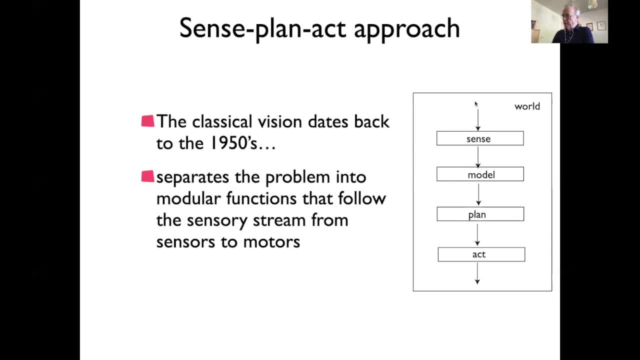 architecture. So, roughly speaking, they had modules of function that would follow the sensory stream from the sensors to ultimately the actuators in different modules And that allowed again to modularize function along that stream. You could say the sense and the plan. 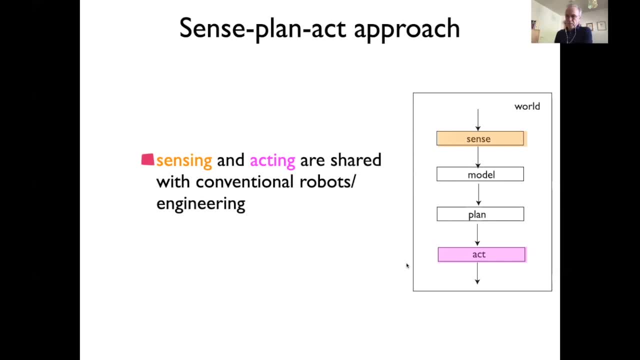 the act part are control and sensory information, signal theory kind of problems that were like in conventional robots or in other areas of engineering, so shared with those not specific to autonomous robotics, While the AI part, the intelligent part, was sort of focused here at the or localized here at the center. 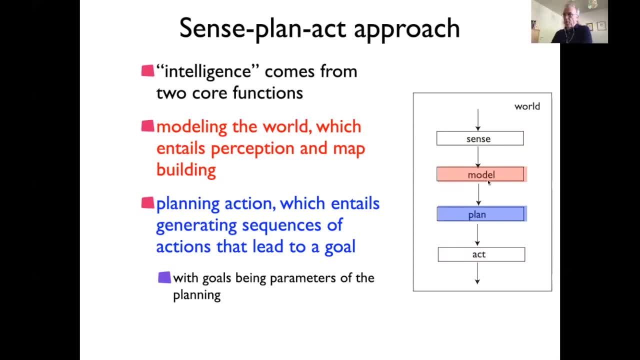 So the model, which would be sometimes called the world model, which is essentially intelligent, is a very detailed perception that is extracted from sense, information, information about the world, and then building maps of the world. in that way, And based on these maps, planning actions. 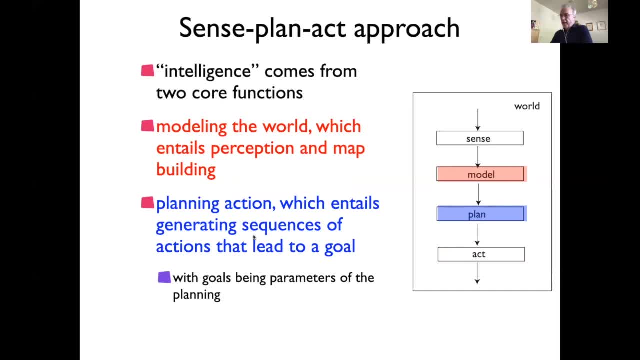 that would interfere, for instance, a whole sequence of different individual actions that would lead to a goal. With the goals, it's not really represented explicitly here where they come from. They would be essentially parameters of the plan And they might have to be acquired from somewhere. 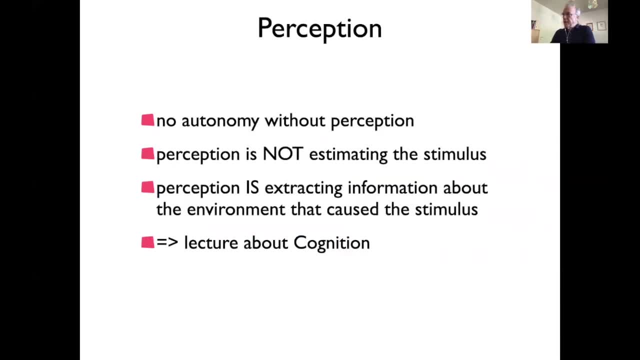 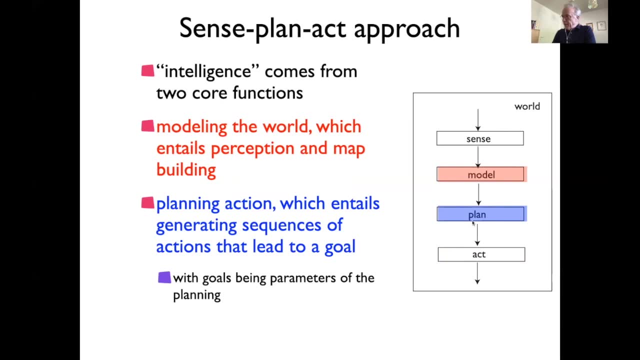 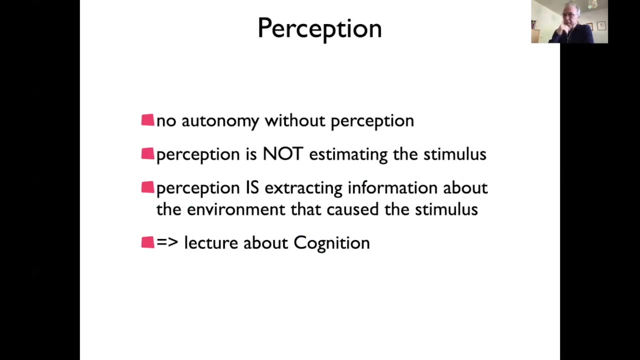 or be set by the program. So I want to say There are a few things about these two levels here: The model level, which entails perception and mapping, and the planning level. So perception is, of course, critical to autonomous robotics. as I defined it, based on your own sense. 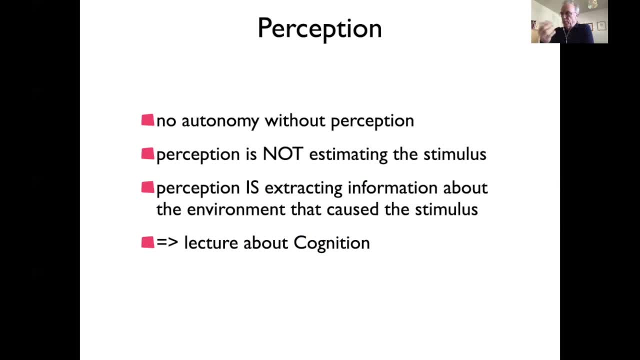 of information and what that actually means, based on your own perception, Because what you do in perception is extract information about the environment. It's not so. perception is sometimes misconstrued as being estimating the stimulus that's going to cause something like image processing. 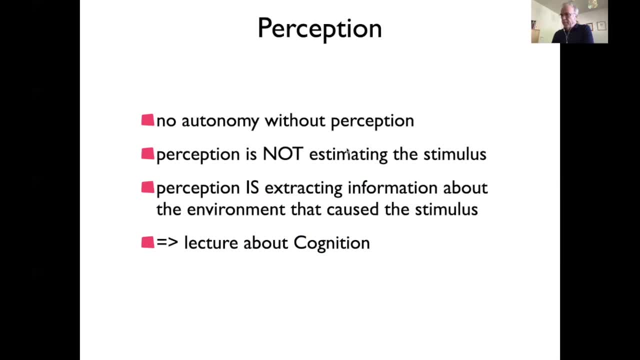 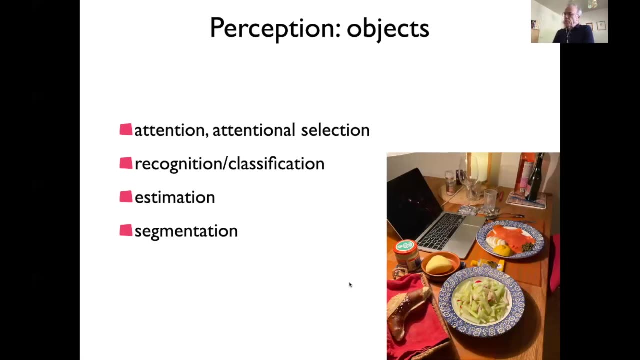 That's not actually what perception is. It's about extracting information about the environment. In my lecture about cognition a couple weeks ago, I elaborated on that point And you might want to remember that. So here, if you look at a scene like that, 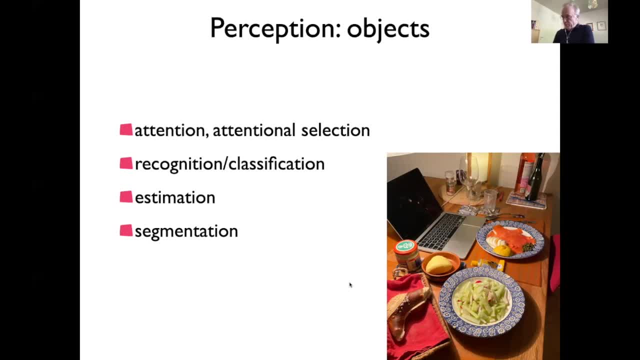 what your perception as a human will be about is about objects. You will be perceiving that scene, maybe the setting of the scene, But you will largely be perceiving the objects in there. And you will be perceiving the objects in there. 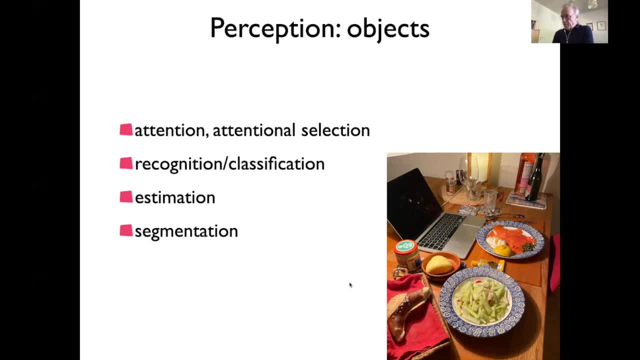 And pay less attention to this picture as a picture, except if you want to maybe paint it or so, So you will, for instance, attend to particular objects, Maybe if you have a task in mind, like you want to drink a glass of water. 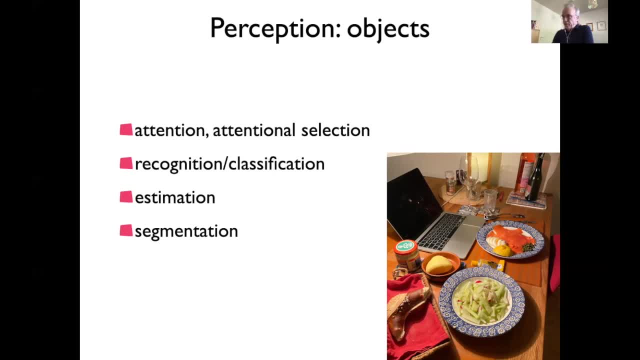 maybe you will look for the water And you will be able to find it in the scene and select that, essentially bring that into the foreground. You will be able to recognize this as a glass and other elements here classified And you might, for instance, see: 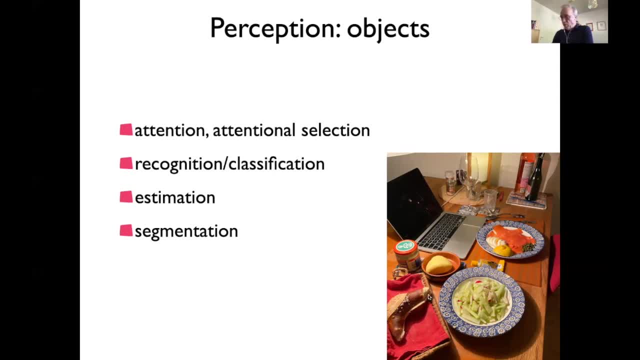 that this is a piece of a pretzel, even though it's kind of broken off. It's not actually a complete pretzel, but maybe you're able to see that, And so that will be an example of invariance under an important form of transformation. 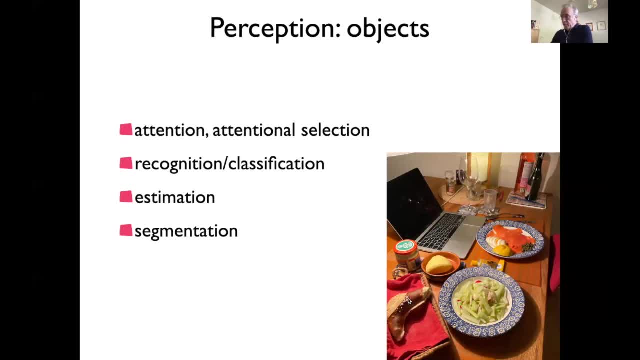 You will be able to estimate things. For instance, you can grasp these objects, And that means you can estimate their pose, compute how far they are, maybe in which orientation you would have to grasp them, and so on. And you will even segment objects, in the sense you will know which. 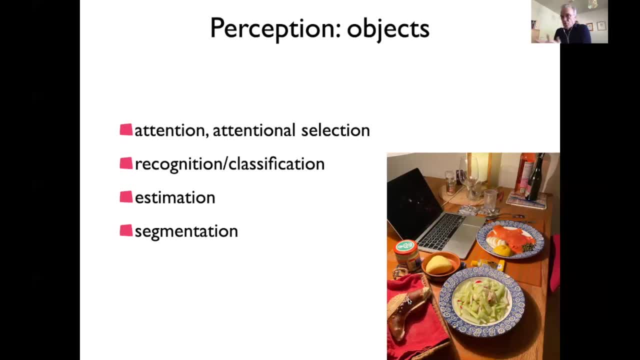 part of the image pertain to the objects and which not, so where the boundaries are in the image. Here this glass is very interesting. You can clearly see this wine glass here, even though it is transparent and uses the visual structure behind it. 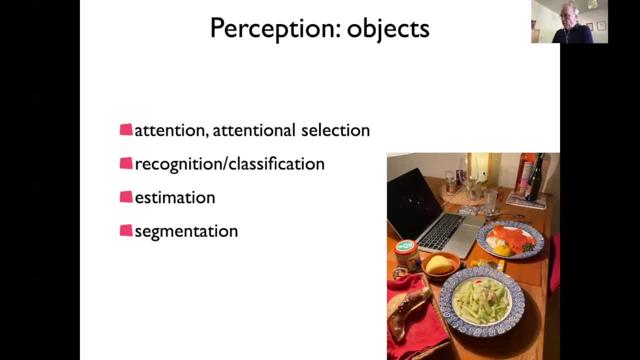 So that's a very challenging segmentation task, to know which pixel here is foreground, which background, because you see the background through the glass. But we are very good at that. That's a real challenge for computer vision. So that's object-oriented vision which. 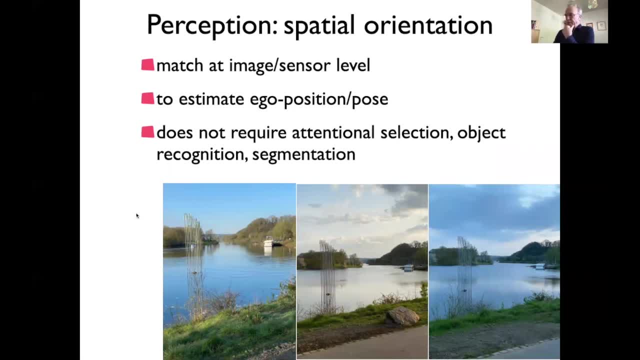 I want to contrast to the kind of perception that may underlie spatial orientation. So, for instance, you could have taken this image at some point And you want to now, when you're there in that same area some day later, use that image to compare it to your current view. 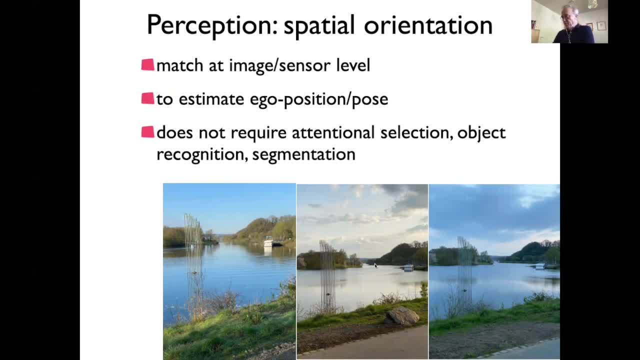 and then say: am I at the right spot? Some of you might recognize where that actually is. And this does involve recognition, matching, namely matching, for instance, different images which are under different lighting conditions, different weather situations, slightly different positions. 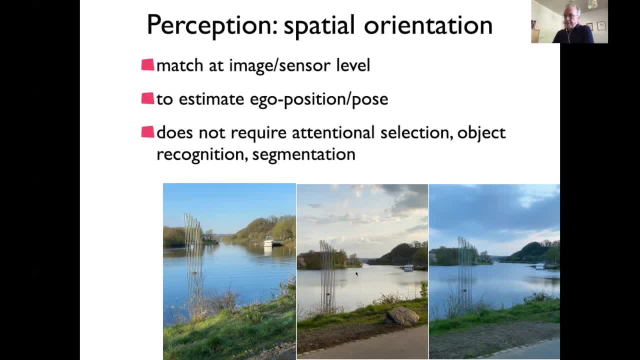 You want to estimate the position from that. So that is ultimately how navigation, estimating where you are- works. It doesn't always work with images. You can have other kinds of sensor readings, often just depth profiles from the laser range, for Andrew, for instance. 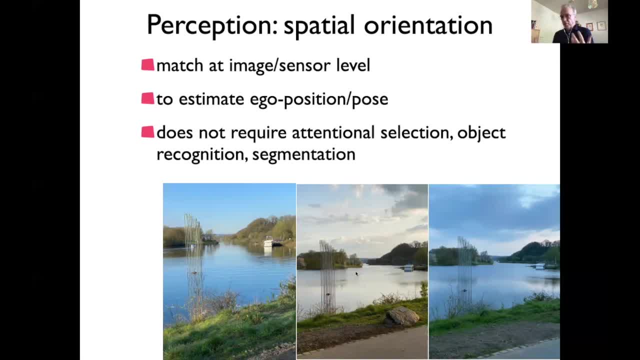 But matching past information to current information to recognize that you're at the same location is the core operation And that's the core operation of using sensory information to estimate your spatial location or orientation. And you see that that requires matching, with some invariants. 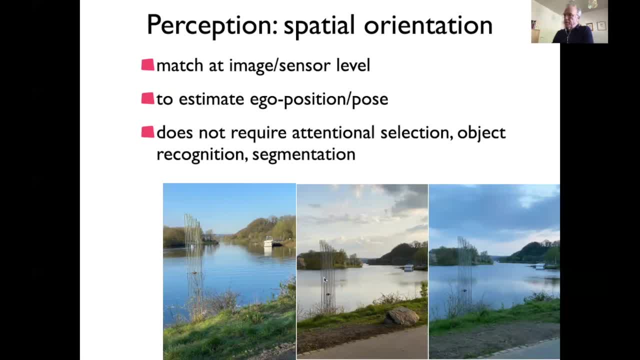 Like here you might have to say, well, this corresponds to that, and this corresponds to that, and so on. So there's some invariants, because it looks different in these different cases because of the lighting condition and some metric transformation, And from that you can then estimate, for instance, your pose. 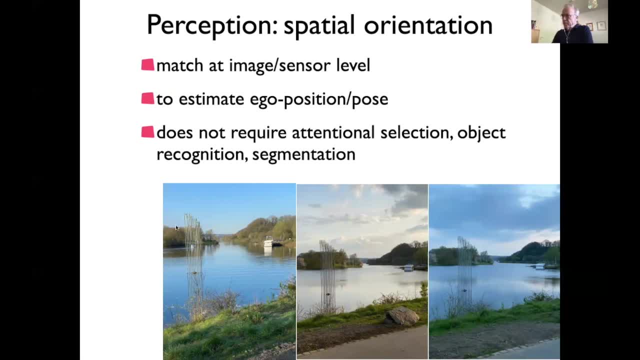 This is a very simple way to do that, So you can have a very simple way to do that, but it doesn't require necessarily object attention. I was drawing your attention to things, but that's just to guide your human performance. But you could do this with just the whole image. 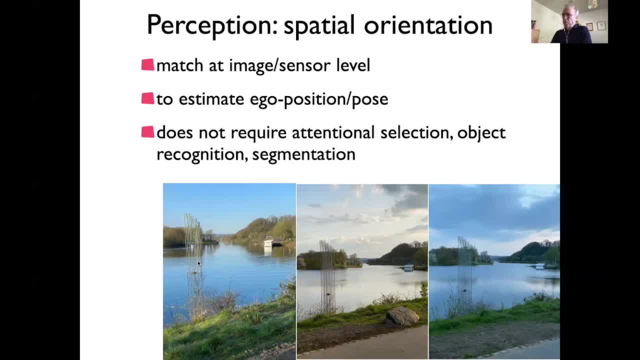 the whole array. for instance, A lot of that is done in navigation of vehicles, where you take the depth profile and just match the depth profile And you don't have to talk about objects in there And certainly you don't have to segment the scene. 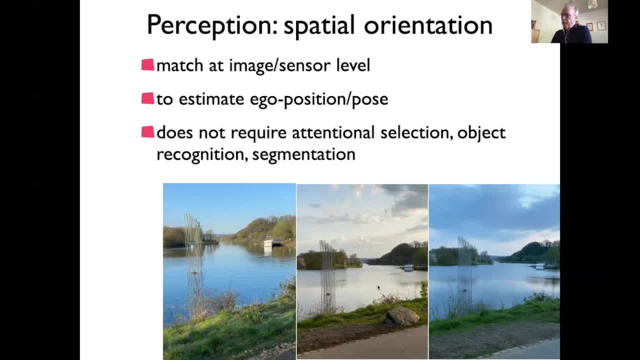 into different portions. You don't have to really say: this is the lake and there are trees and so on. So the demands on perception for essentially estimating your ego position are quite different. as you've seen, They are actually less or less sophisticated. 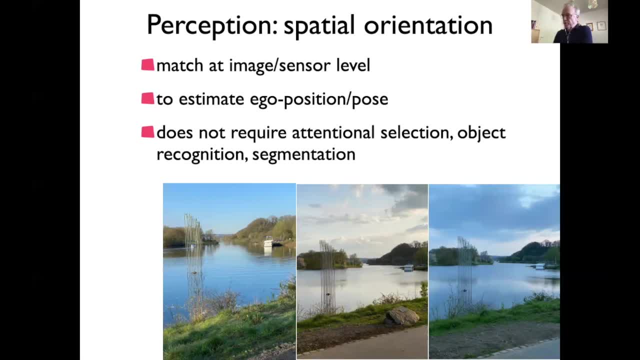 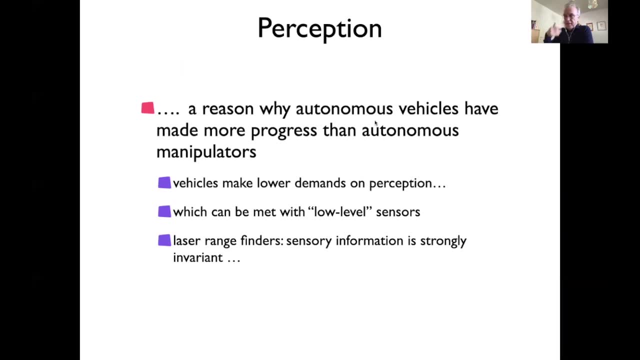 They are things that lower animals do and that simpler algorithms can do, And that is one of the reasons why autonomous vehicles have made more progress than autonomous manipulators. So manipulators are actually orienting the action at objects, while vehicles essentially just need to know where they are. 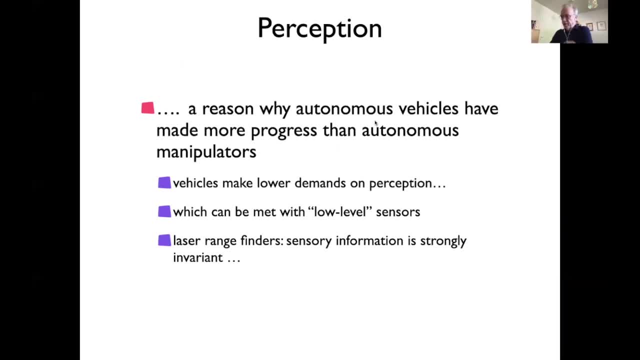 and then they might have to, And that's why you need to do a little bit of object orientation, in the sense of maybe seeing the road, But you can even navigate based on just a compass and a direction. So a lot of these demands for orientation. 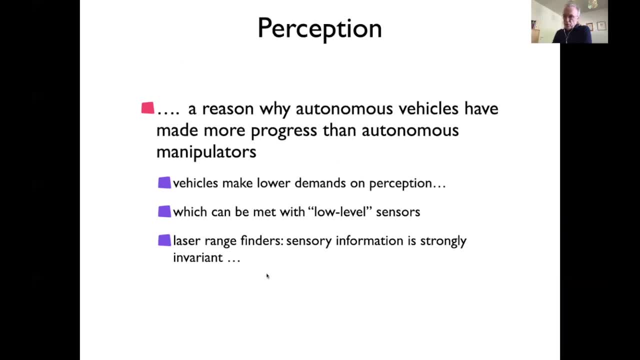 can be actually met by low-level sensors. Distance sensors are often considered them. They are low-level In the sense, for instance, just a single signal, the depth signal- But- and maybe in terms of their ecology as well, when they're 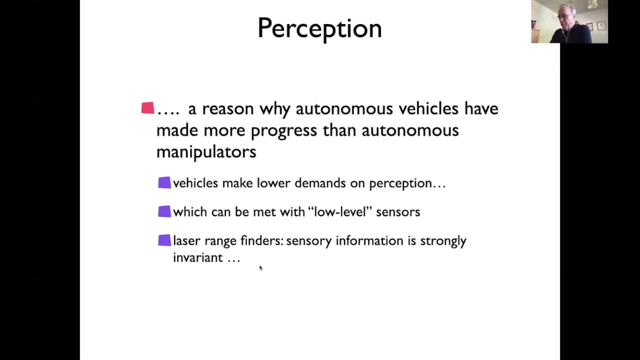 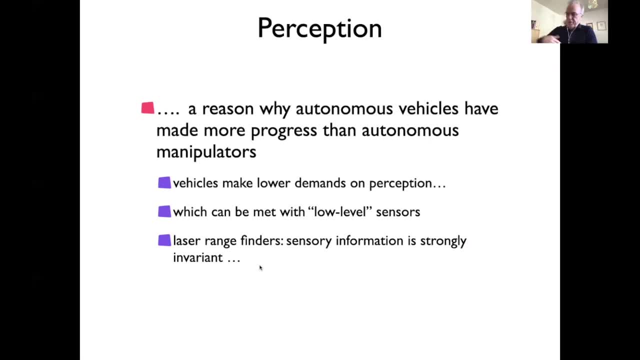 they are actually also very invariant. That is, if you're at least in a range finder, it will tell you the distance, no matter what material or what the lighting conditions are or the weather is and so on. So that's been a big source of progress in the vehicle domain. 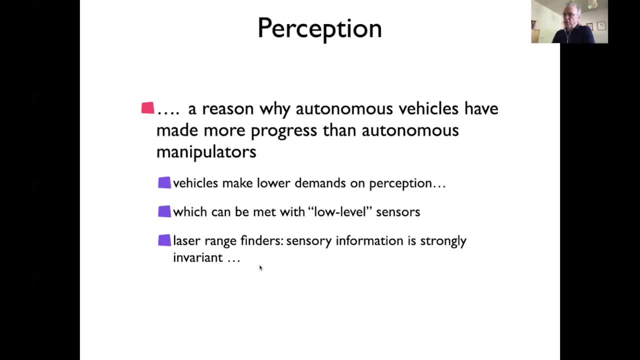 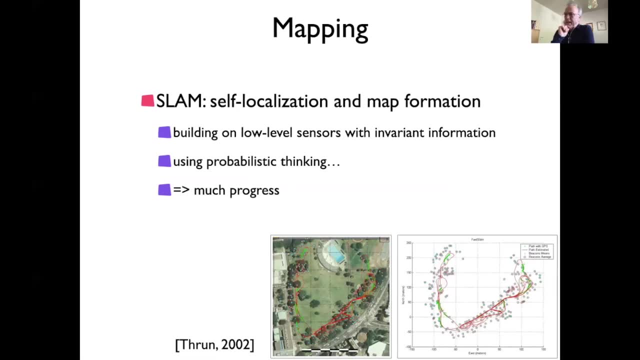 that when, with low-level sensors, you were able to solve these orientation problems. Yeah, maybe that's here. There's a famous problem called SLAM, self-localization map formation. that essentially it's a very complex problem. that essentially it's a very complex problem. 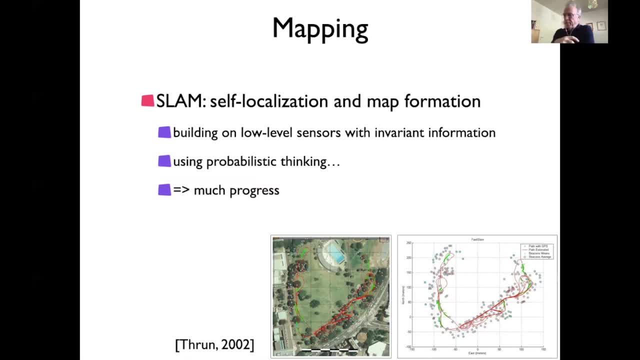 that essentially, it's a very complex problem That actually combines the map making with this form of estimation. So what you're trying to do is, as you drive around, you're trying to take your low-level sensor information, store it and make, therefore, the locations at which you acquired. 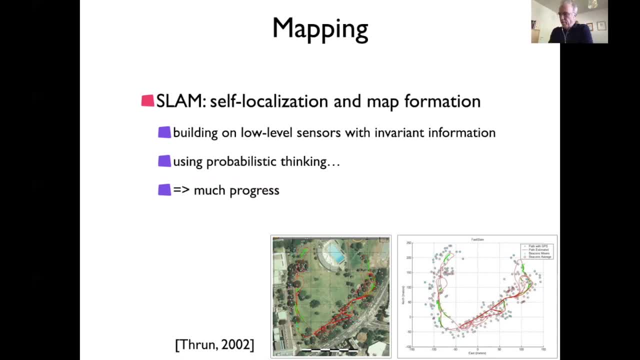 it recognizable when you come back to those locations And from that you want to build a map yourself, while always the mapping based on your own estimate of where you are, And that's been an area that's made a lot of progress, essentially through what is called 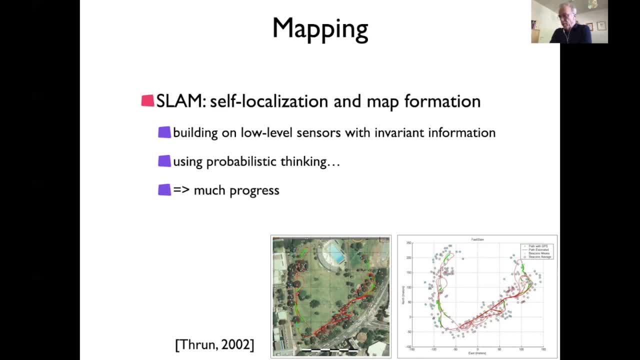 probabilistic thinking or probabilistic methods, which I'm not going to elaborate on in this lecture. Sebastian Thun is a famous researcher in that area. There were actually a group of three German fellows: Dieter Fox, Sebastian Thun and Burkhardt. 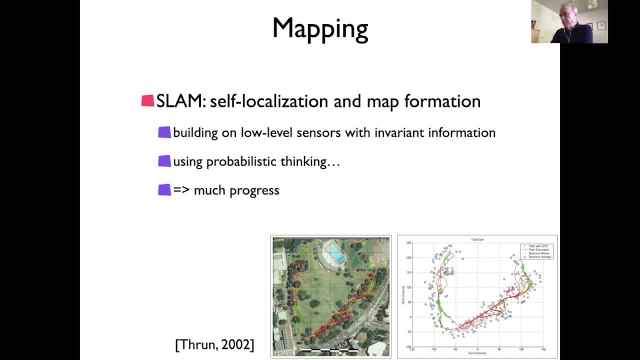 I can't remember his first name- who made a major contribution with these probabilistic approaches and pushed that field far ahead. So some people even consider that soft. There are a lot of practical problems to how to actually pull that off. This has very large demands on storage. 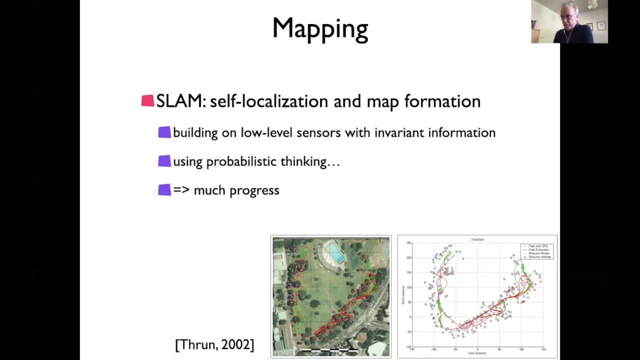 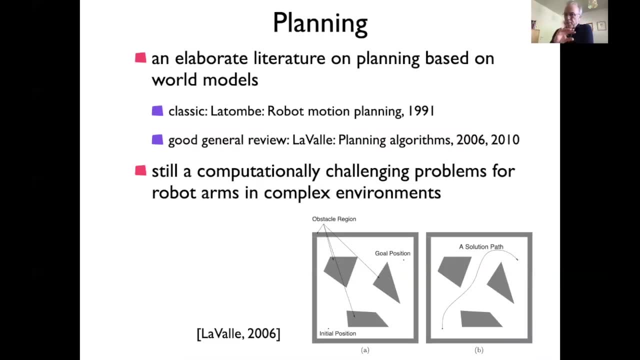 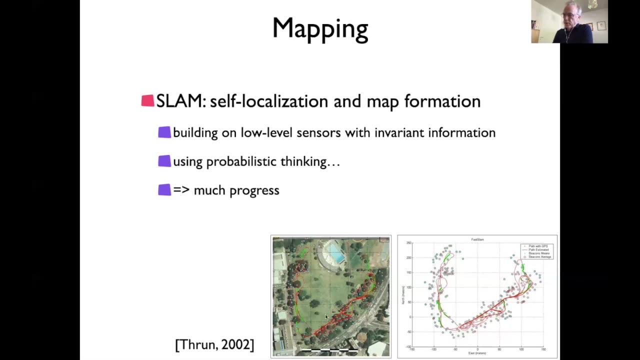 and in some cases on computation, But there's considerable progress in this area. So much about mapping and perception. Last, what I want to say that the more extended idea of this would be that what was called a semantic map, that is, at different locations in the map, you also 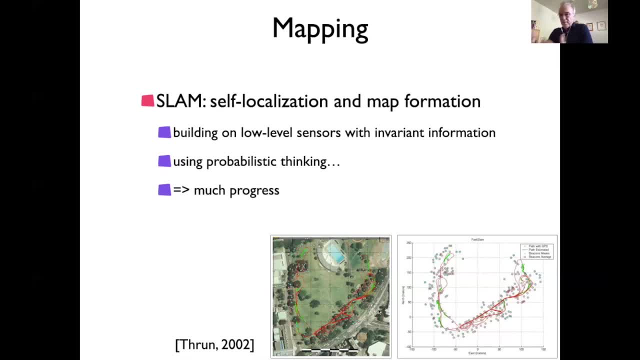 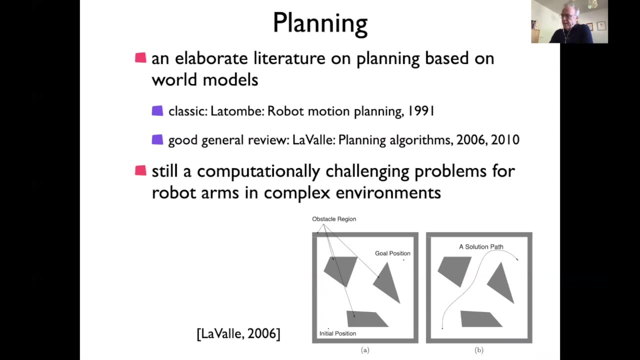 recognize objects now and really acquire meaning, therefore about the objects, And that of course entails these much more difficult problems, and that's a topic of cargo research. So planning is an interesting field. There's a lot of literature on mathematical methods. 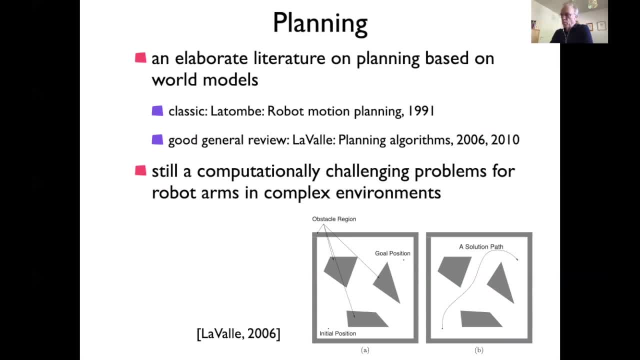 of planning that is based on having world models, often world models that are mathematically idealized, for instance, like these polygonal surface maps where you would describe Objects and areas in the air, and like polygons, which is difficult to really obtain. 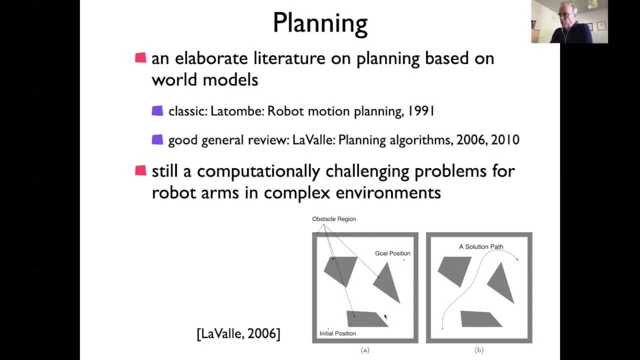 from sensory information, But if you have it, they're very good. mathematical approaches: Classical, it dates back to the 90s and early 2000s. Some of these are computationally still expensive to achieve. So achieving, solving a path in higher dimensions. 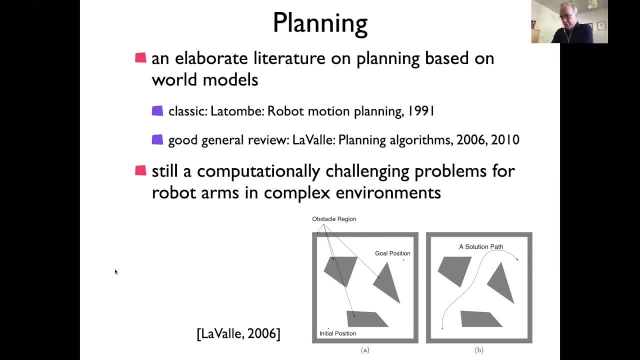 when you have a complex robot arm problem can be computationally demanding, So that even today to do that in real time can be hard And some people build special purpose processors to solve motion planning problems. And motion planning is still a very active topic of research. 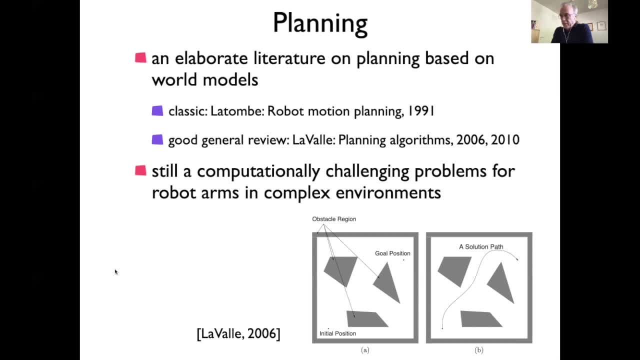 At robotic conferences you will have, often the largest sector of contributions will be in the motor planning, movement planning domain. But I would say it's a well mature field with a lot of techniques And its problems are largely having that world map. Tobias Glatzmacher has lectured about an aspect of planning. 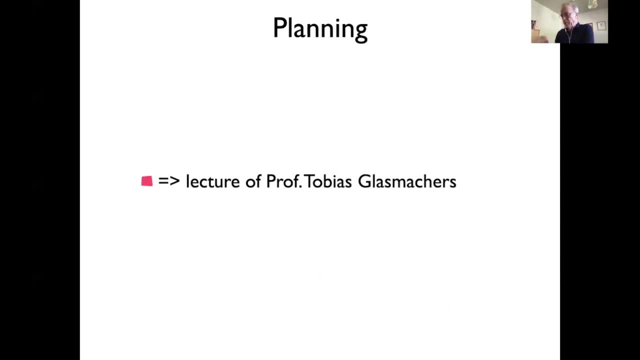 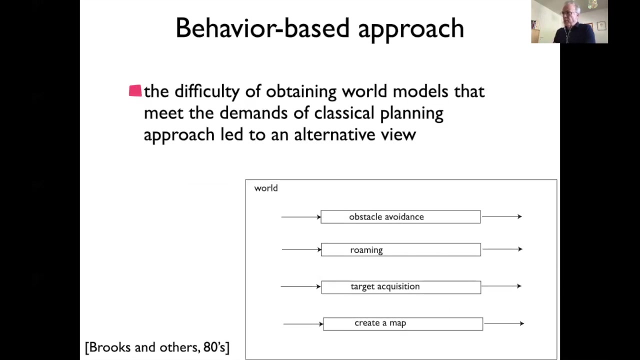 which wasn't exactly path planning, which is sort of like a sampling of that literature. This is important: AI literature, For instance. a lot of this is using search algorithms, minimization of some kind and then reinforcement mining, So I don't want to go deeper into that. 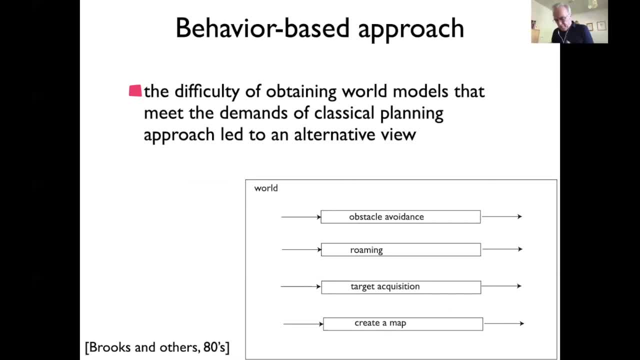 But I want to say so. this was all in sense, plan act picture. I want to say that the major difficulty for that has been the obtaining these. This is all about the So in the 80s, late 80s and 90s, an alternative approach. 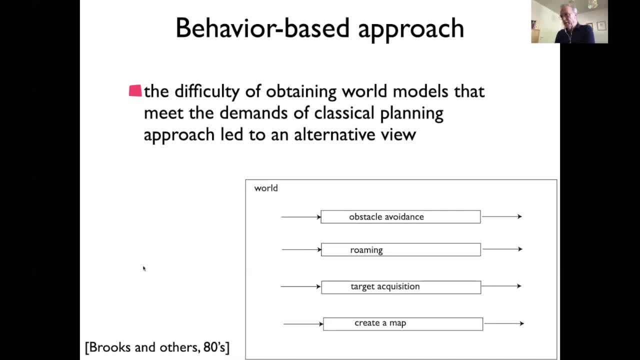 was developed. It's not a single approach. It's an alternative way of thinking was developed That sometimes runs under the name, under the label, of behavior-based approach. There's different forms of that. I'll mention Ronald Arkin in a moment. 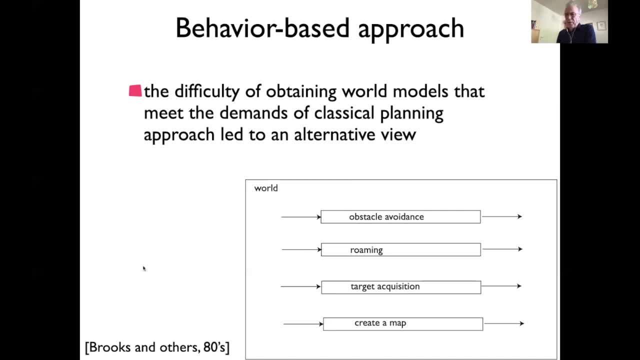 So the idea was we need to get rid of that world model. And one problem with the world model is that it is sort of general that all the behaviors can take the same world model And say: instead, in nervous systems we see there are specialized behaviors. 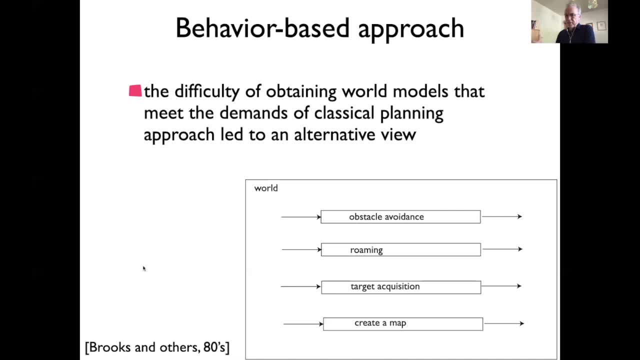 And these behaviors have access to special channels of central information. It's actually even in the human- you could say for instance, what and where system in some sense, And so, for instance, information about spatial location orientation is achieved by a special path that doesn't actually 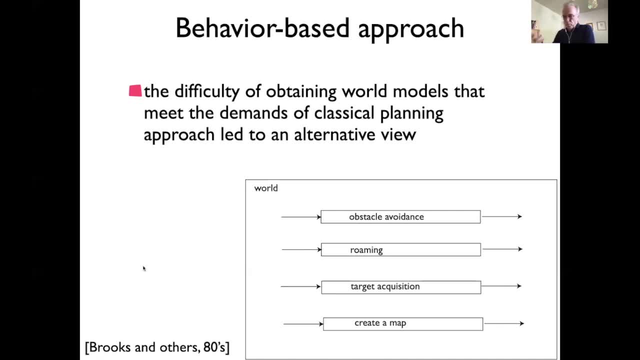 have the same complexity as the path that supports recognition, for instance, And so, in this view, you would build the robot from a bunch of different behaviors And each behavior has its own special purpose, sensory input and acts on motors, And they would be quite complex. 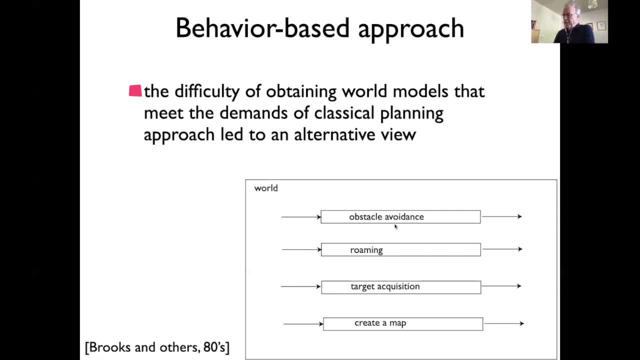 They're quite restrained with respect to how they interact. In some proposals they can only activate each other. Sometimes they can what is called subsume, that is, to provide the input to another module or get the input from another model. behavior sorry. 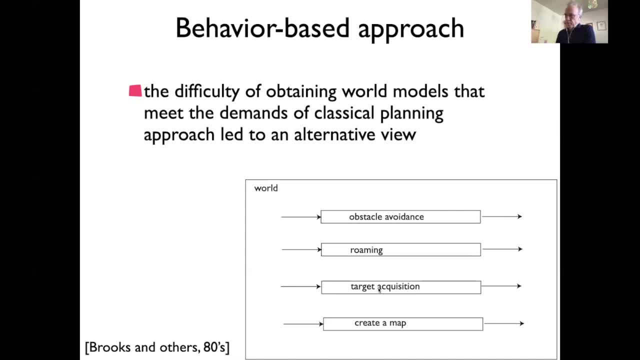 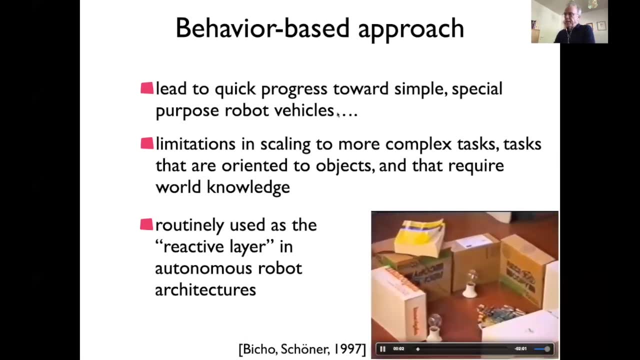 So to avoid to have the same architecture problem again just between these objects, And that is I mean. it was a very successful approach. It led to a real breakthrough in that simple special purpose robots became feasible with simple sensors, And these examples of the robots I showed you. 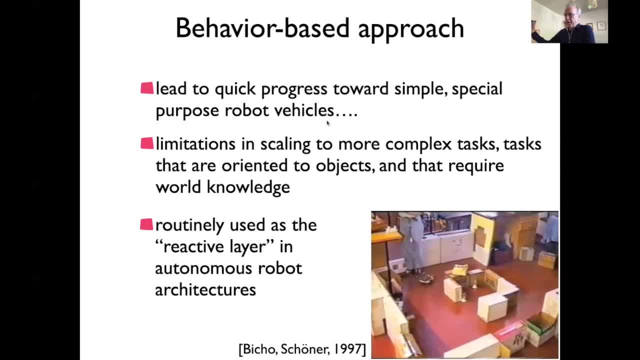 at the beginning. the simple special purpose robots you can buy in any electronics store now or in a commercial store. Those are all sort of inspired by these kind of ideas, even though they are now already much more complex than that. The limits of that also appeared quickly, that is, they do not. 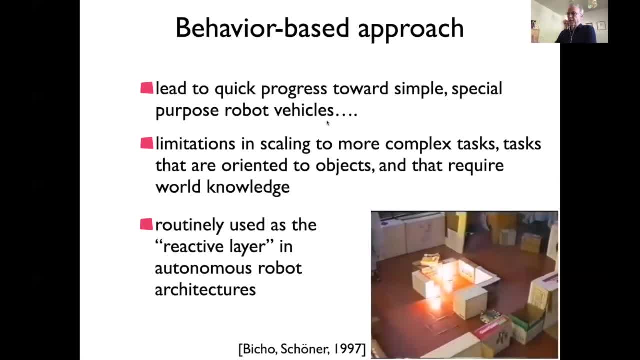 really scale to more complex tasks that require longer term planning. especially, they are essentially just basing- usually the behavior on the sensory information immediately available And that's why they are something called reactive And so they don't have really plans. This is actually a little demo that we did a long time ago. 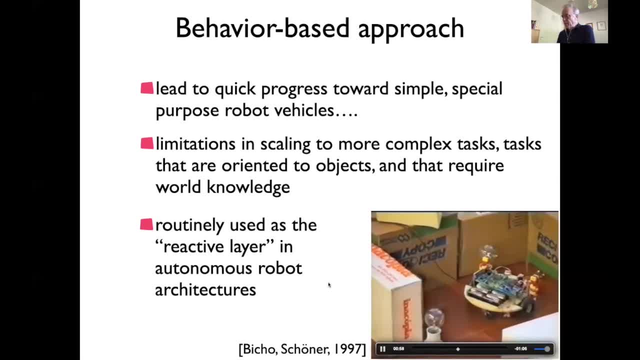 The electronics of this is the Lego robot. It was at the time not yet available from Lego. It's an electronic kit one could put on one's own little robot And it's an example of a robot. But that is extremely simple in terms of its internal algorithm. 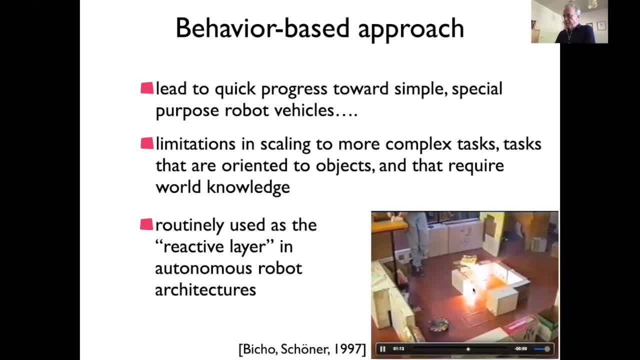 It's based on dynamic systems, but in an adequately structured environment. it seeks out sources of light in a way that looks intelligent in some sense, But it's all just reactive. It's very, very low level. So these kinds of approaches have not gone away. 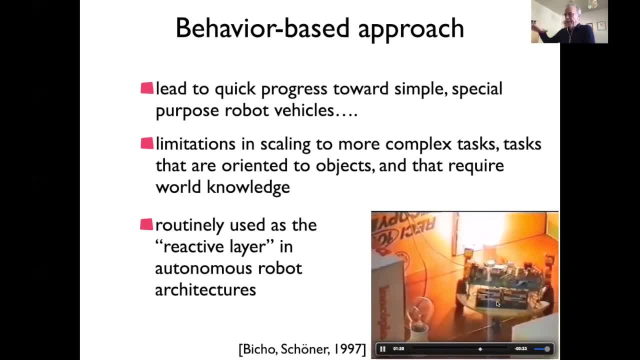 They are very influential as sort of a basic level, sometimes called the reactive layer, of robot architecture. Very many approaches Use those And they essentially say that for the fine control locally of movement, especially of vehicles but also of arms, we will rely on special purpose sensor information that solves. 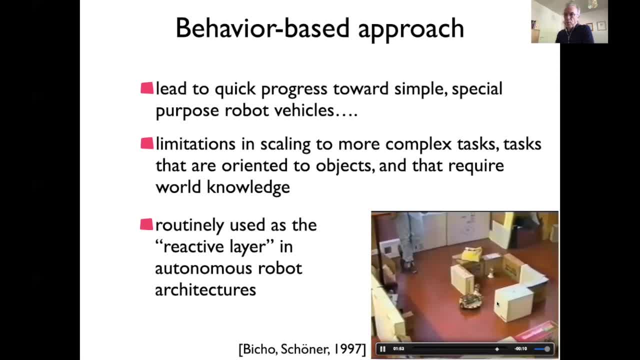 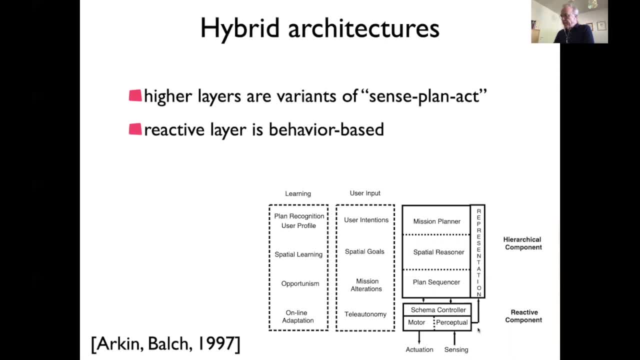 these tasks in a very special way and not rely on having a world map of everything. So here's an example from an architect, who's also older, where there is a reactive layer that we call schema control, But sort of the same kind of idea. 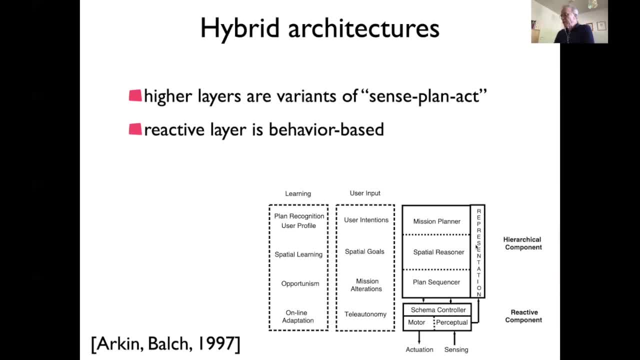 And then there would be more conventional sense plan act systems with also learning and user interface components that then act onto the robot through that reactive layer, And that's very common. It's sometimes called hybrid architectures because it combines these so-called sub-symbolic and the sense plan act kind of approaches. 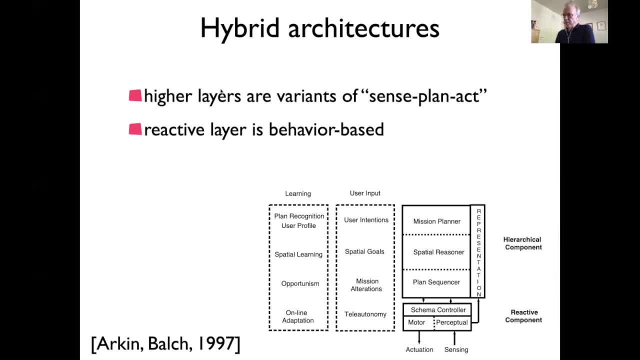 And that's sort of the state of the art today. You will have many systems like that, And a lot of the autonomous driving algorithms actually have some kind of architecture Like that of reactive planner and then planners at longer and longer planning horizon and that make more demands on sensory information and mapping. 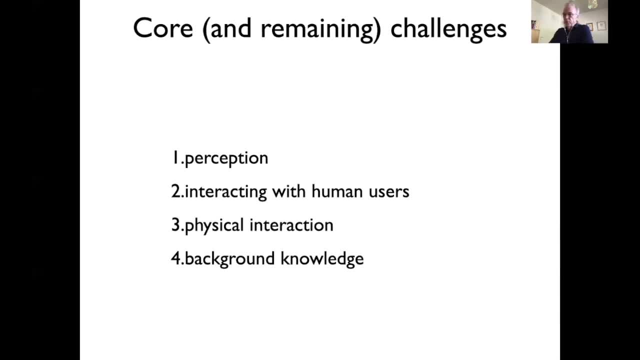 Good. So I want to close or come to the end of this video by talking about core challenges that remain challenges- Some of those I already mentioned- but they remain research challenges that really similar to what autonomous robots can really do, And they are very interesting research challenges. 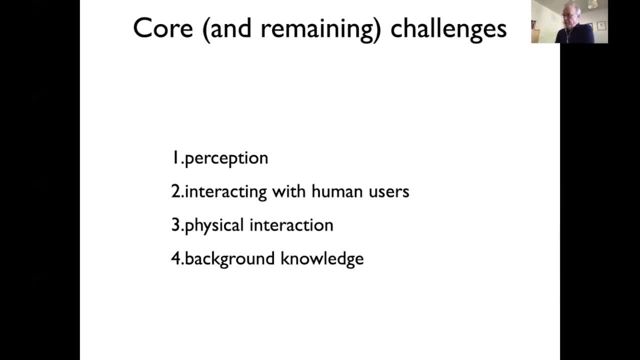 So I'll mention four of those, two of which are very related. So I already mentioned perception, of course, And I say it was originally the big crisis. the world sense plan act, the world model was just so hard to come by. still frontiers. 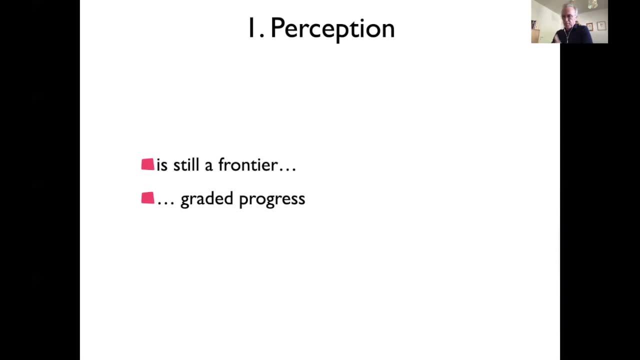 The progress has been very limited. I mentioned the vehicle domain. There are these special shortcuts, much simpler there, but in object-oriented models it's still very limited. So I want to talk a little bit more about that. But in object-oriented action, which 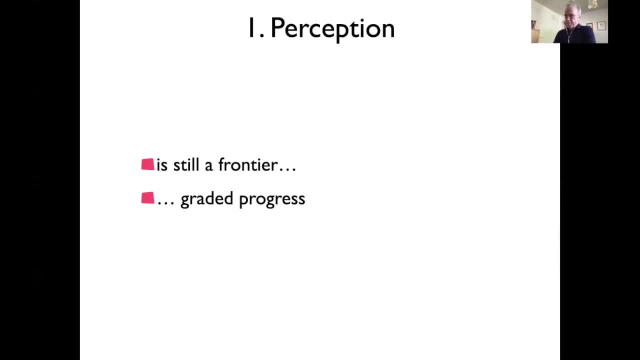 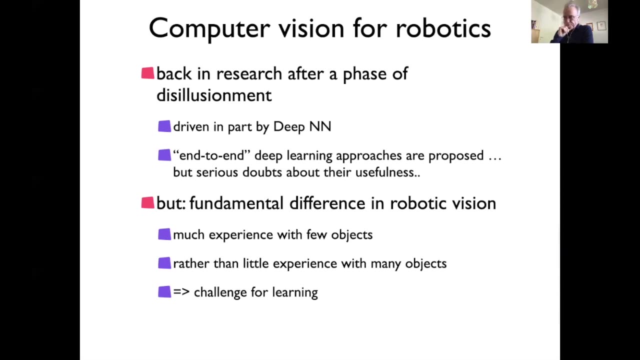 is the basis for more interesting behavior. this is still a frontier, So there was a period when computer vision was not used much. This was when the laser range finder, the vehicle research was very successful. But people have come back, partly because computer vision. 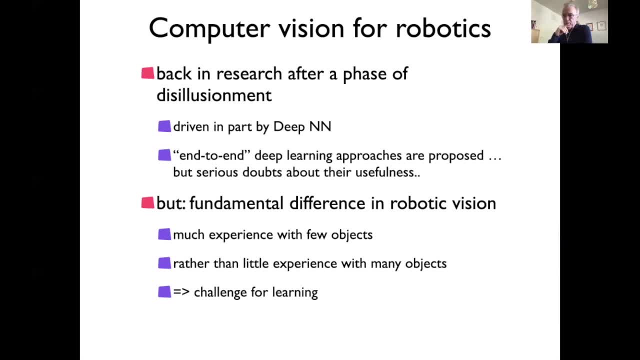 has made a lot of progress, in part based on deep networks and other machine learning approaches, in part also just because of the scaling of computing power, And it's generally on learning ideas. Currently there's a lot of so-called end-to-end deep 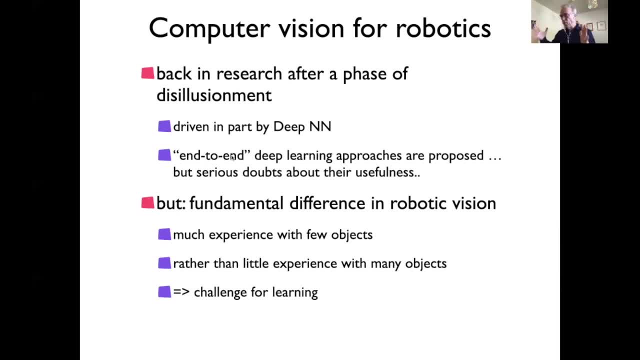 learning. So we take just raw images and you take some raw control output and just brute force learning with a lot of time and resources. That is being criticized in the robotic community about its lack of usefulness and the invariance, But since, when you change the visual environment, 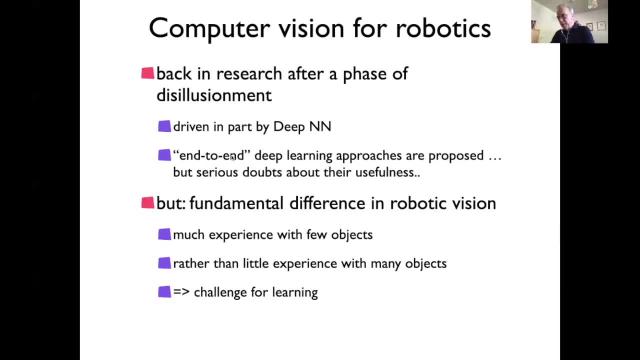 you don't want to relearn all the control and so on, But there's certainly a strong research enterprise in that direction. There's one fundamental need: There's a fundamental difference between robotic vision and a lot of the computer vision that is used in strong alliance. 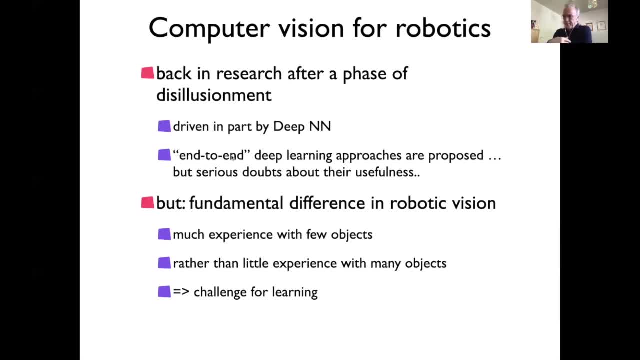 with machine learning in that in robot vision, you typically have only a limited set of objects in your working environments. The classes of objects you deal with and maybe the complete exemplars will be limited in nature, But you'll have a lot of experience with these objects. 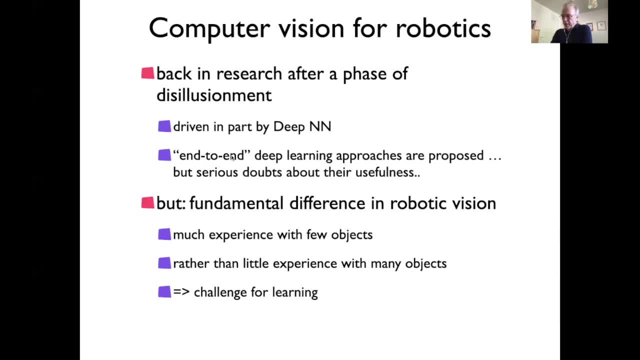 While a lot of the computer vision algorithms they're based on having limited vision. they're based on having limited vision, They're based on having limited experience in just single images or small clips with many, many, many different objects, And these many objects would essentially 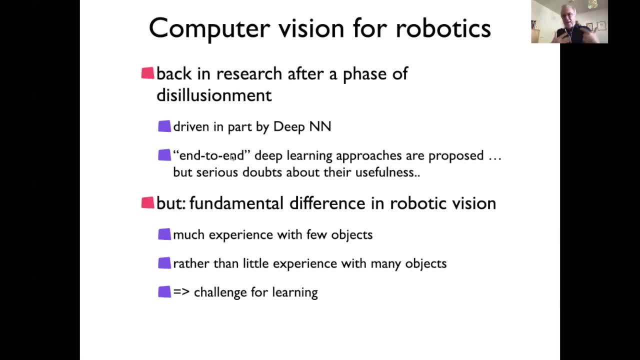 explore all the variance and then you extract the invariant component that helps you classify and maybe estimate, And that means that the assumptions of these groups are not necessarily valid in the case of robot vision. So that's one of the challenges, for that I don't want to go too deeply into that. 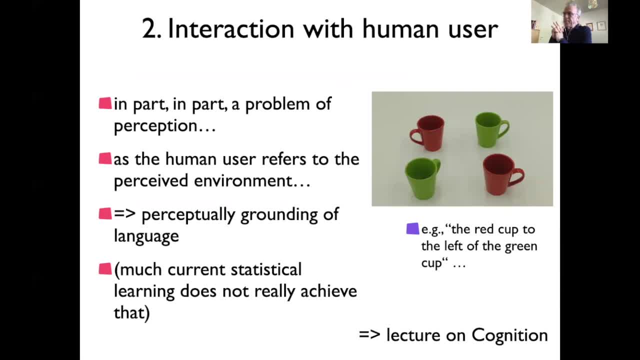 I mentioned that interactivity. I mentioned that interactivity. I think that we should. I think that the ability to interact with a human user overlaps in part- Sorry, I have that word twice here, Overlaps in part with the problem of perception, in the sense that 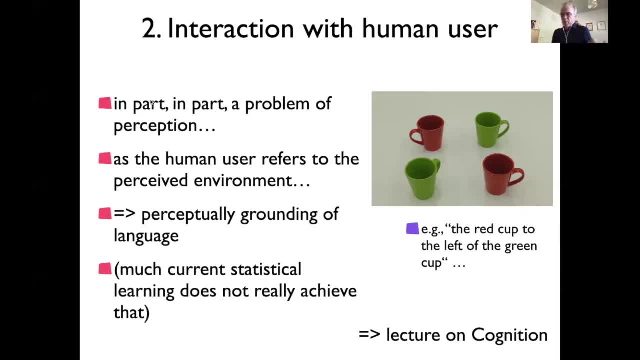 when the user interacts with a robot, interacts about that shared environment and refers to that environment, for instance by language or pointing or other things like that, And that will mean that the robot has to perceptually ground the language, And that's harder than one thinks. 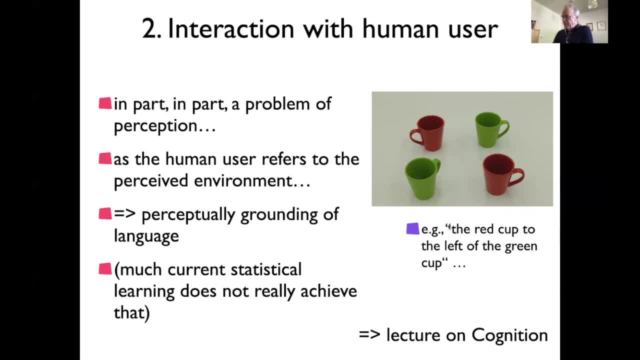 In my lecture on cognition I did elaborate on this example on showing how cognitive that is, how you have to potentially test hypotheses and reject some And there's a real understanding of world properties to do that And it's a bit misleading in part in that computer vision. 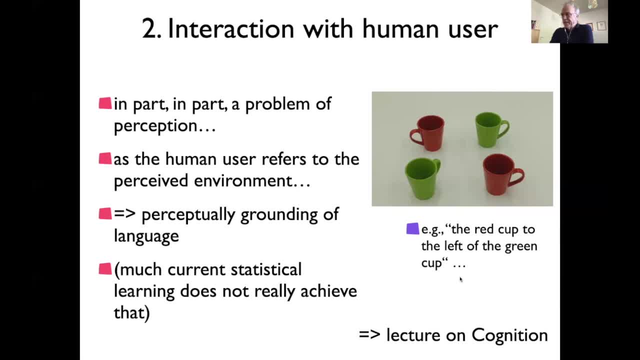 with machine learning has achieved things like that. For instance, Google does all this work on searching for images by typing in words, and it would then be able to find images that match those words. In the past, they were very trivially just based on matching to words. 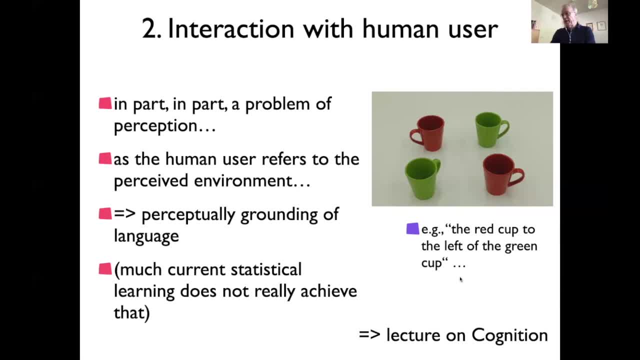 that were around the figure in the source where that figure came from. But increasingly they have algorithms of how to analyze the images and associate them with words. But that still doesn't mean actually that these algorithms know what they see, They know about the world. 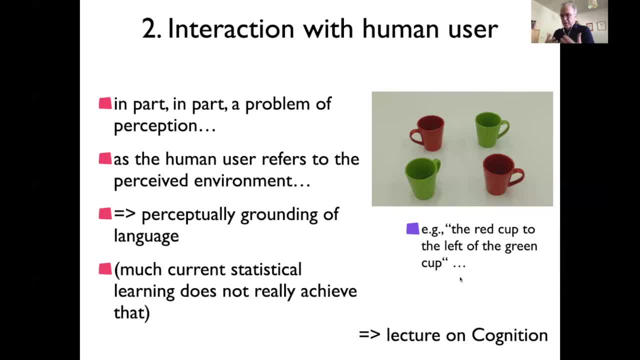 They just find some associations that certain images are best associated with certain words, maybe certain parts of images as well, And so this is a challenge and there's a lot of work on that, For instance, attentional algorithms, things like that. So it's an interesting field. 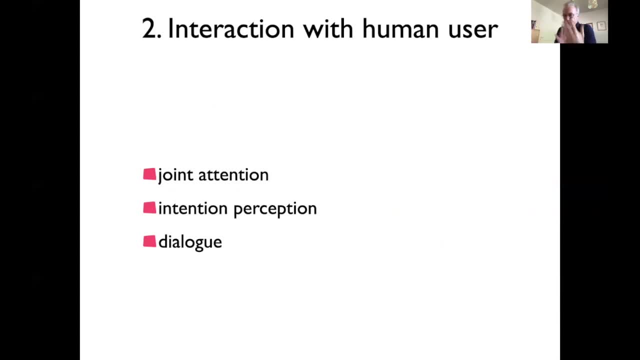 And of course then there's also the aspect of- so that's just the perceptual aspect of grounding language and language being supportive of communication, And then you have to do things like understand what the intention of the user is, and that's partly a linguistic problem. 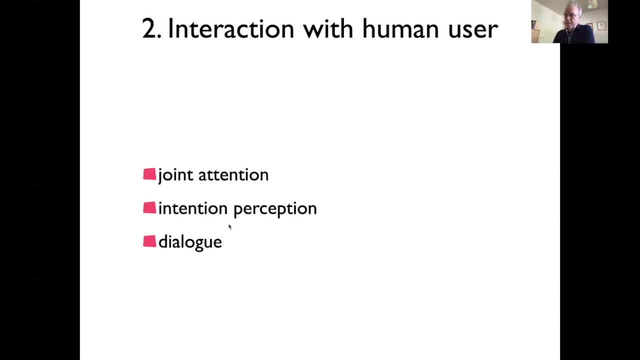 understanding the meaning of sentences and the pragmatics and what the user wants, And partly there is some form of embodiment in here in that there is user, the user tends to something. you might want to find out what that user is attending to, based on gaze. 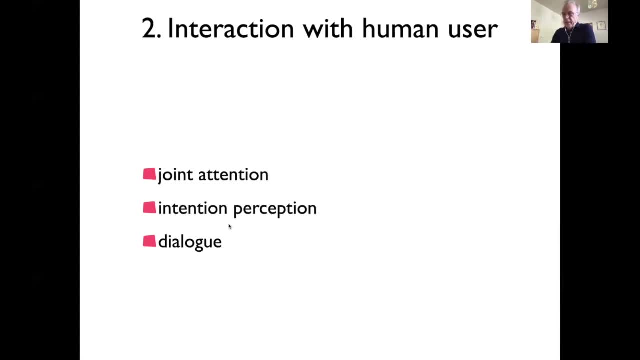 maybe based on body posture, based on the recent history, predict what the user is going to be about. And then there's the whole aspect of engaging in dialogue, of actually real communication, And there have been a lot of demonstrations of systems that fool a human into thinking somebody does dialogue. 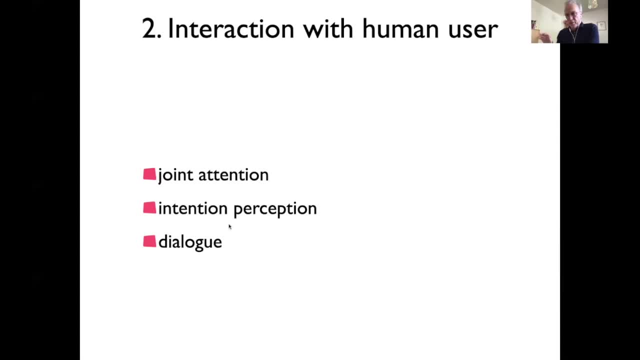 but that's just scratching the surface because that's just sort of playing. but doing a dialogue to actually achieve something together, to work toward a goal, is actually quite subtle And a little challenge for you if you ever work with someone like you don't know how to do it. 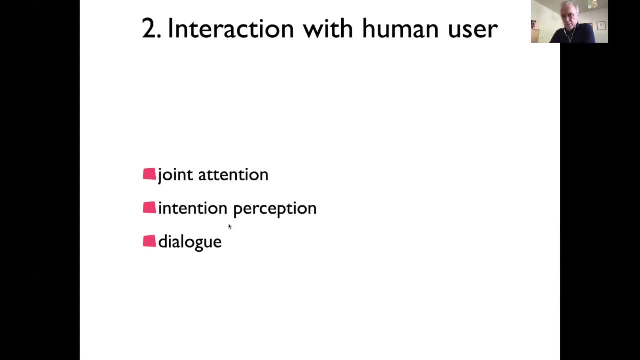 You don't know how to do it. If you load a truck, let's say you're moving your apartment and with you know, with someone you carry the furniture, pay attention to what you're doing. That is amazing how much communication there is physical. 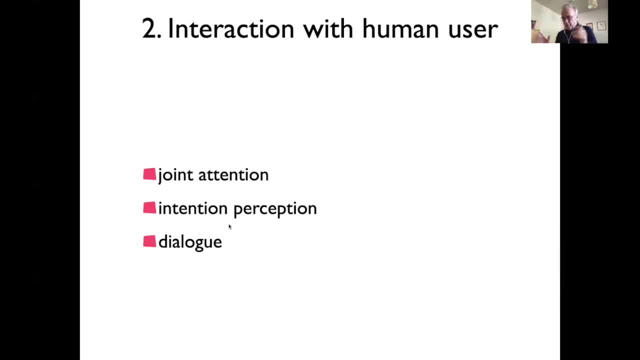 where you don't have to explain exactly how to grasp the couch and how to turn it, where there's a lot of looking. you look at a place and the other one knows: ah, that's, I have to look at that corner and maybe lift that up. 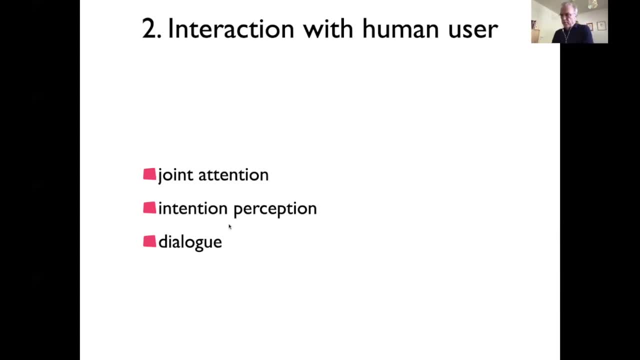 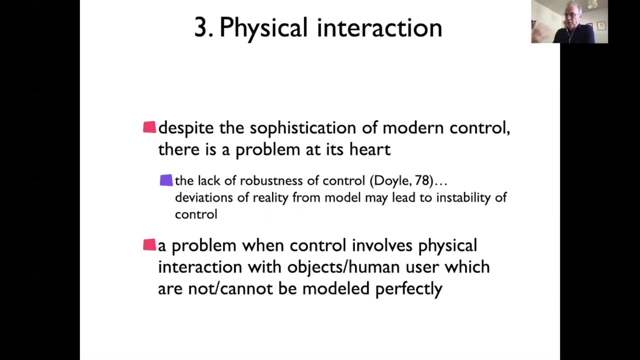 or by your body posture, you suggest a certain way of doing things. It's very interesting. That is very hard to emulate. There's some serious work on that Good. This entails sometimes physical interaction, So for instance, jointly acting on an object with a human. 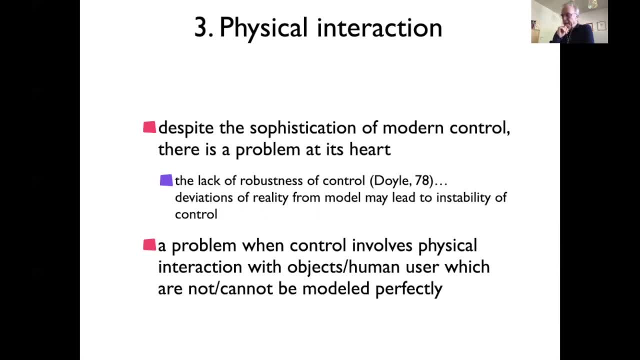 or actually directly physically interacting with a human, like guiding a human and so on, And that is a big research frontier. that is not so related currently to machine learning techniques, even though maybe it could be, And it's a little misleading sometimes, you know. 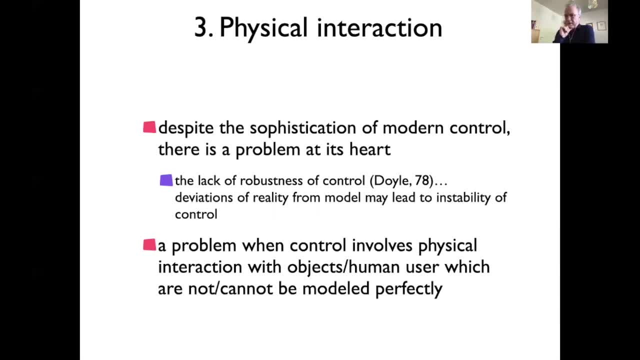 modern control theory is very, very sophisticated. It's mathematically very well elaborated and with modern computing can be implemented And in some sense an enormous level of sophistication. but at its core there is a problem. It could be summarized as the lack of robustness in control. 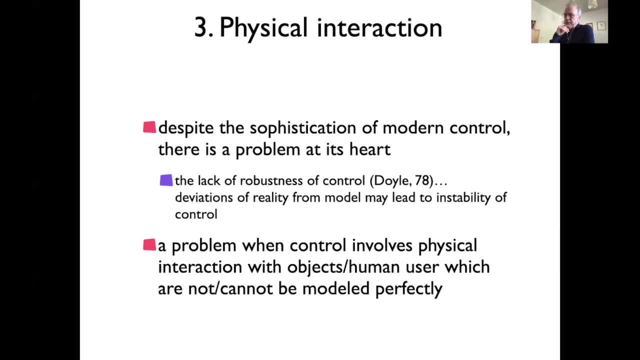 It goes back to a theory that comes from the seventies that essentially says that if you have a small deviation of reality from the model, there is always a possibility of having an unstable control system. So you cannot actually give a limit beyond which you will always have stable control. 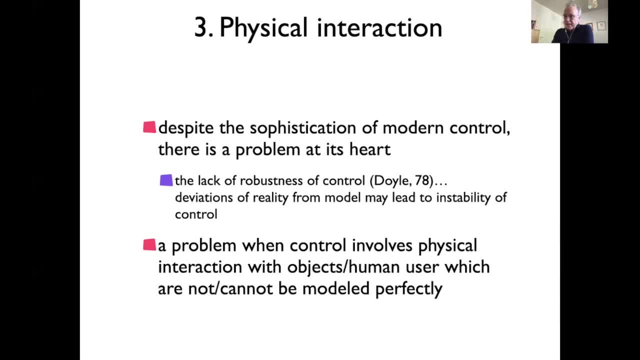 And that's a problem, because when you physically interact with objects or worse, with humans, and then your models are going to be perfect, If you're an autonomous robot, right, And then you'll be interacting with objects that you only partially know, and human users are notoriously difficult to model. 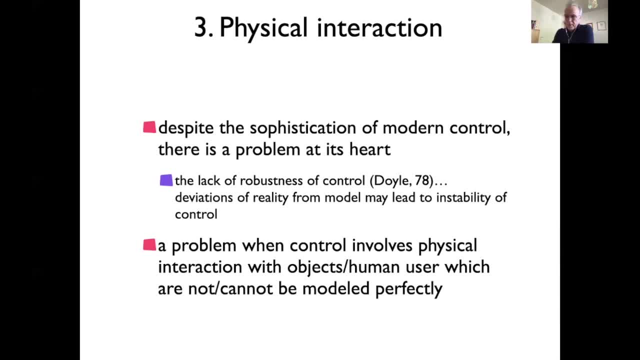 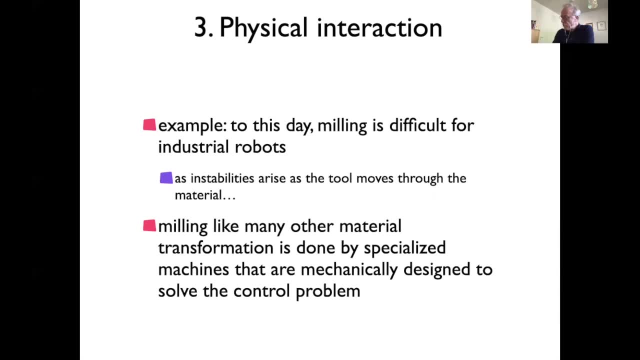 So you're likely to run into these kinds of robustness problems, And they are not just academic problems. For instance, a lot of people don't realize that all these robots in industry, they do a largely contactless task or the contact is very limited. 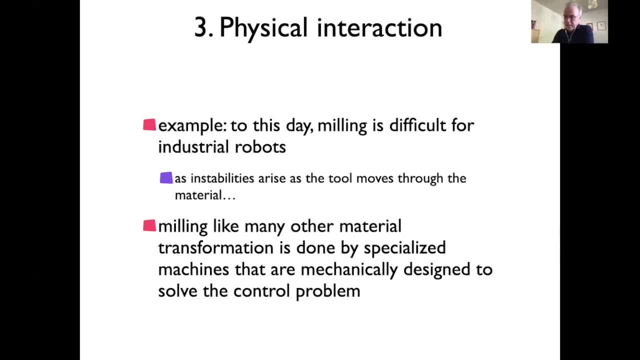 For instance, just grabbing some hook or doing something simple. They are not doing things like milling right, Where you have to have an interaction with the surface and take off a little piece of material in a well-defined form. And the reason for that 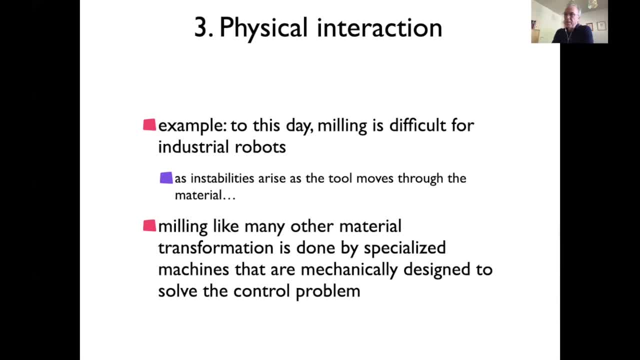 is that very typically, robots go through instabilities as they interact with material like that, For instance, because of the difficulty to control forces or control torque, which is very difficult to do, And so many of these machining operations are done by specialized machines. 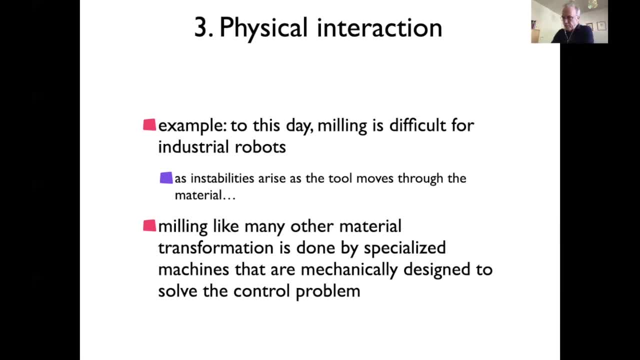 which are not robots in the usual sense of articulated arms. This means these are specialized. They are mechanically designed to solve the control problem. The German machines- the machining industry is famous for developing all these very specialized machines which they can sell all over the world. 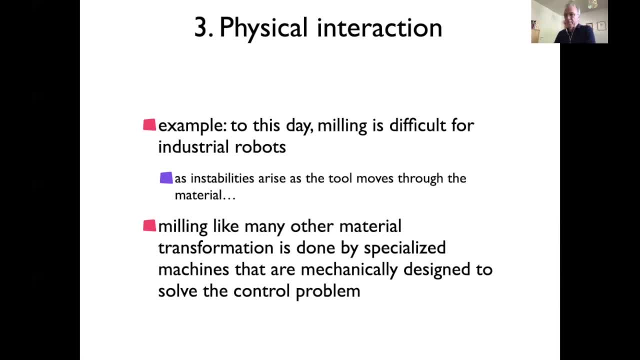 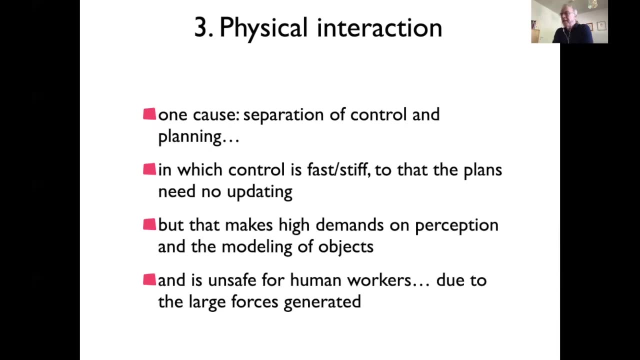 And production companies would be happy to replace them by robots, which would be much more versatile and flexible, but that's very hard because of these control problems, And so that's a real problem for autonomous robotics, And if you look deep inside, it is ultimately due to the separation. 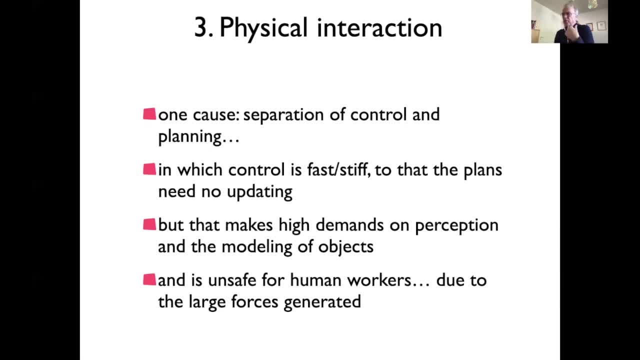 of planning and control. So control is so successful because it is fast and stiff in some sense. So it makes it keeps the error, the deviation from the plan, very small And that makes it possible to keep the plan, just have a plan and just track it and not need 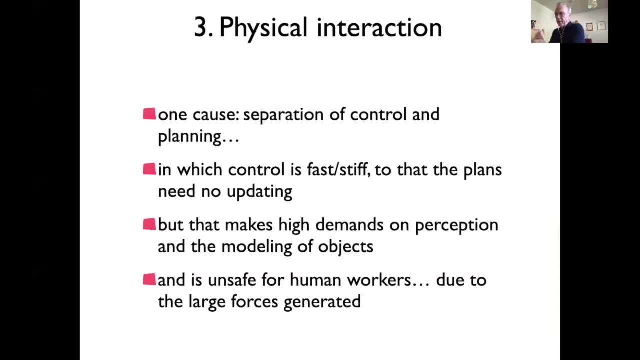 no need to update the plan because the error was so large. you now have to re-plan And that makes these high demands on perceptions of the models. have to the plans have to branch. For instance, if your plan is slightly off, like you're trying to plan a posture. 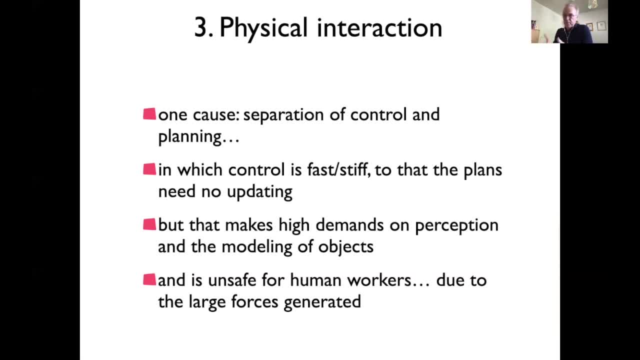 that is slightly inside the actual, then the robot will destroy the object because it's trying to do it with all force to make the distance from the plan posture small And if it's kept by interaction with the surface from doing that, it will keep ramping up its torque. 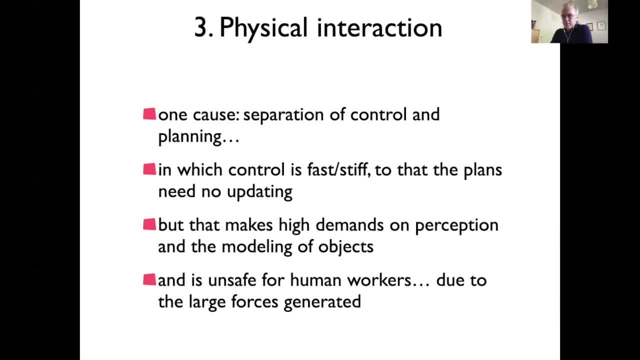 until it cracks the object. So that also makes these robots very unsafe for humans because of these large forces that are generated in order to keep the error, the deviation from the plan so small. So in a way, the difficulty of physical interaction is really inherent. 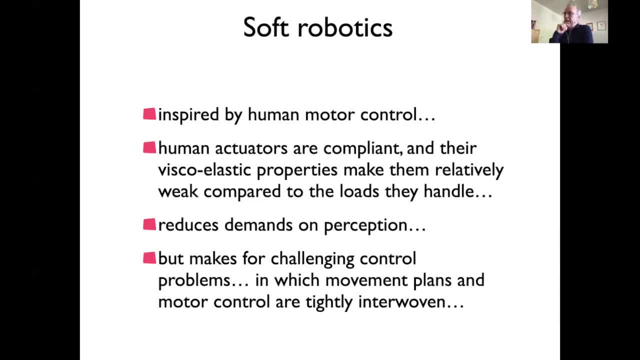 In the approach that classical control takes. So an alternative that is currently a hot topic in robotics is sometimes called soft robotics, which one I think is inspired by human motor control. Maybe not everyone, maybe it was invented independently. It's certainly true that humans, as robots, are soft. 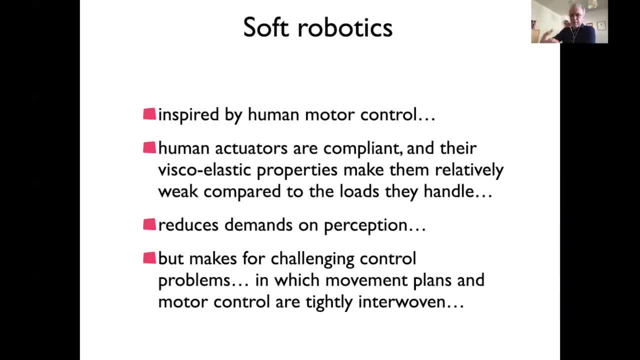 They are soft in the sense they are compliant, viscoelastic. the muscles are viscoelastic. They're essentially damp springs And not, I mean actually other. all robots are damp springs in some sense, but they're extremely stiff, while the muscles are relatively non-stiff. 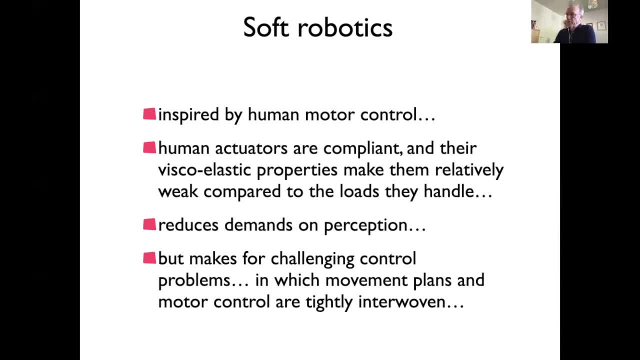 compared to the loads that they can handle. So when you stand upright, you know you're on an unstable pendulum, right, You would fall over. It's the muscles- that's, you know, on both sides of the body that keep you up. 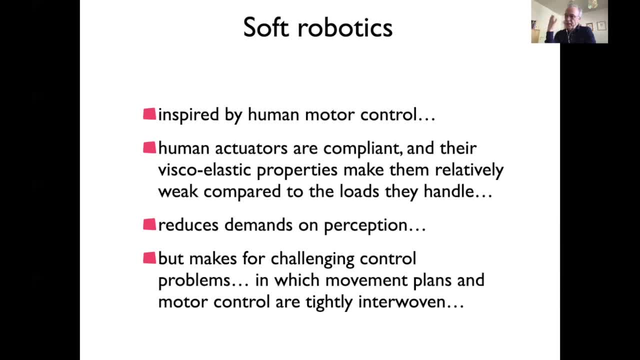 And these muscles are so spring-like and you could think, if these spring are strong enough so to be, You know, to compensate for the inverse pendulum, which is sort of a spring, mathematically speaking that is unstable, then you know. 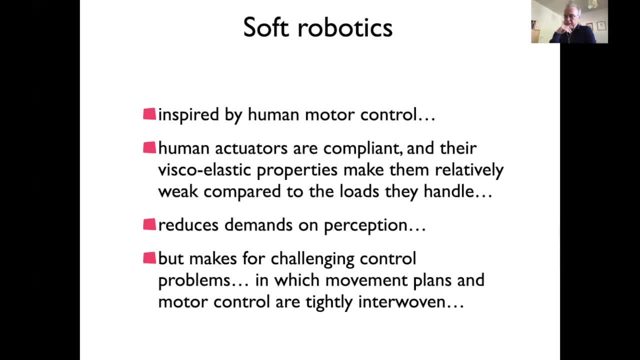 that would stabilize upright posture. It turns out that the muscles are too weak for that, So what you actually have to do is to send active commands all the time to the muscles to keep you in this balanced position. That's a problem that a classical robot. 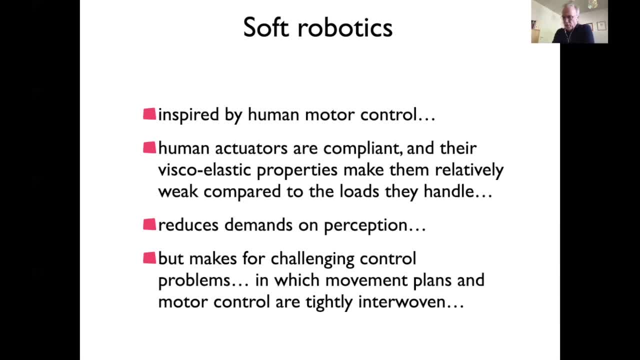 like the ASIMO Honda robot doesn't have because its joints are so stiff by control it can just passively stand there and will not sway and not fall over As long as the center of mass is over the foot surface. So when you make actuators compliant like human actuators, 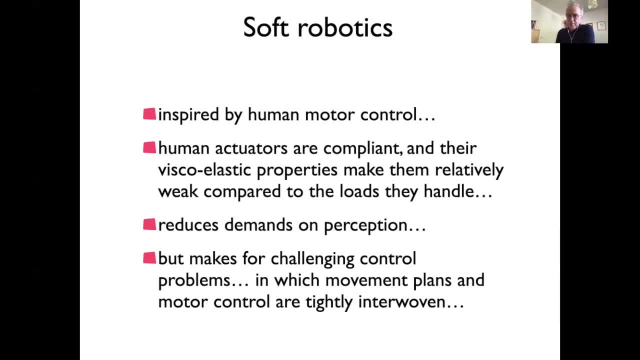 you can do that by adjusting control mechanisms or by using physically, like springy actuators, some robots that have little springs inside and tendons, and they would usually wrap up the tendons rather than contract to, you know, to charge the spring more or less. 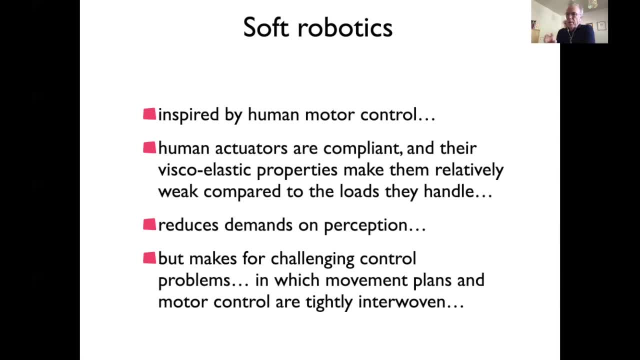 And you know, come away, you know avoid destroying objects. So they don't need to know as much about an object once you grasp a glass. they just need to plan a posture somewhere inside the glass and the spring and all the actuators will then create the force. 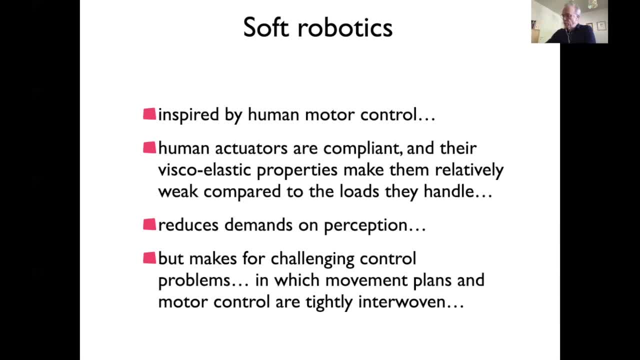 the compression force that will allow you to hold the glass, And so it doesn't matter as much if you've estimated the surface of this glass so precisely, which, in the case of a glass, again, is one of the harder problems, right? 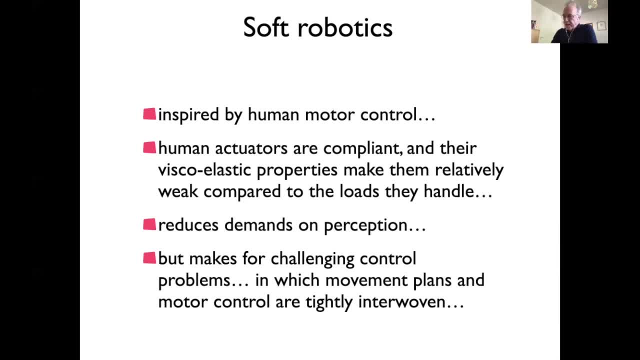 Now the downside of that is, if you achieve that, then you have a problem with just regular movement without objects. you know, making a fast movement with a arm that is so soft is harder, you know Now it's, you know the arm might overshoot or oscillate. 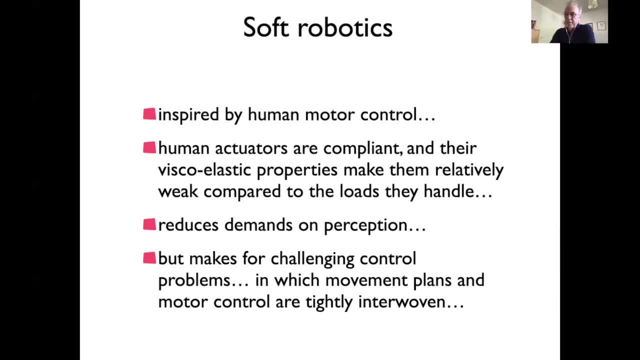 and you have to have very good temporally structured plan that are just right to make now reasonably fast and precise movement. And that's a topic of that kind of research- how to do that. And that's based on the plans and the control. 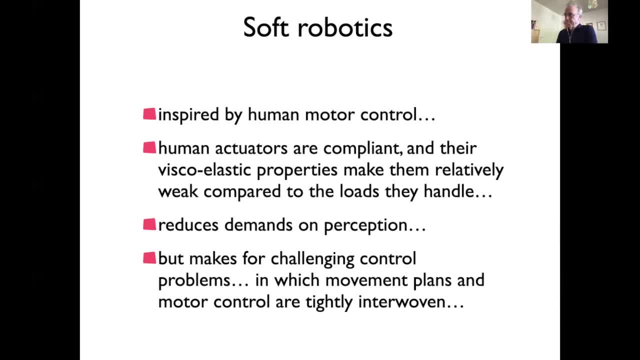 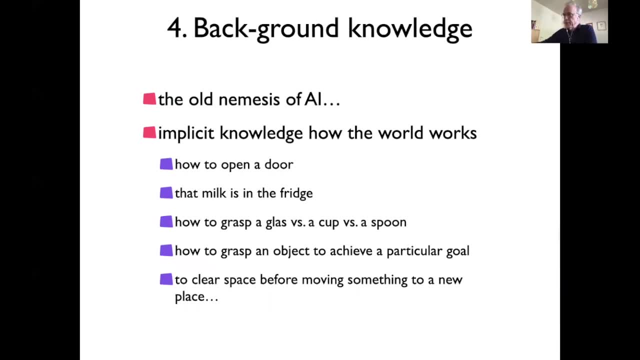 being much more tightly interwoven and more interdependent. So that's very big area of research. Final topic: background knowledge. It's actually the old nemesis of AI. One of the big, big problems of classical AI is how to get world knowledge. 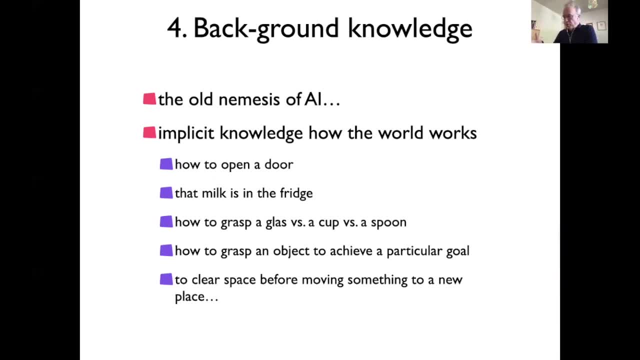 into these intelligence systems, And the classical approach was, of course, to represent knowledge by rules that you could invoke, And it's very hard to code everything you know about the world, or you need to know about the world to achieve a task in terms of rules. 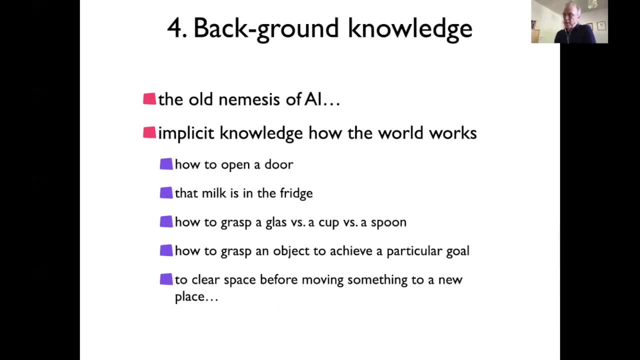 And that's particularly true about robotic action, because that entails a lot of world knowledge that is graded, is fuzzy, is not precise, So it's very difficult to formulate as rules. you know how do you open a door, How you know where is the milk is in the fridge. 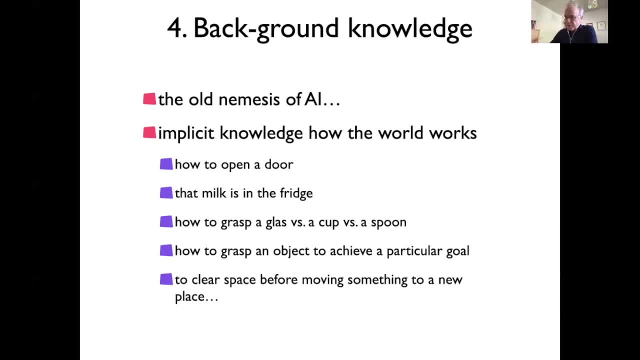 how to grasp a glass versus, you know, maybe a plastic cup versus a spoon, and how hard to press, how you know what kind of grasp will allow you to then do a certain kind of action. You know, putting something down. 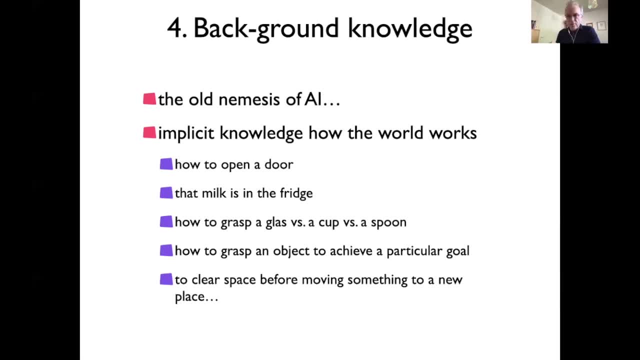 that you have to clean the space you know, and how large an opening you have to make to put an object inside. You can imagine the number of things you need to teach your robot. It is large and amorphous and difficult to formalize. 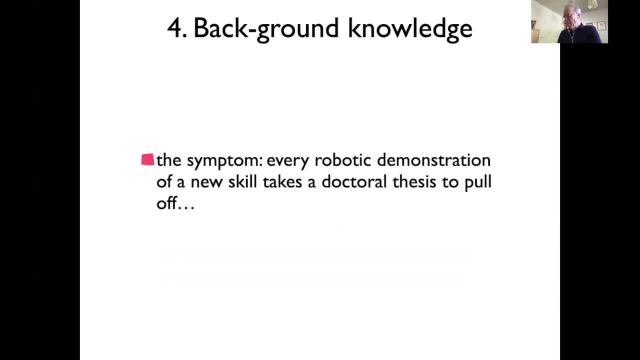 So it shows up very practically as the problem that whenever you have a robot demonstrating a new thing, like a cooking robot that you know makes an omelet, that's a whole doctoral thesis to do that right. And then if you next week try to make a steak, 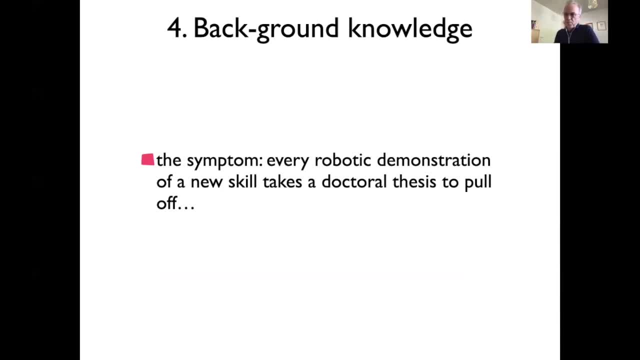 then you have another doctoral thesis, roughly speaking. So there's a problem there, And if you look at robot demonstrations that are around, they are still underwhelming. If you look at robot soccer or look at the DARPA challenge, you'll see that. first of all, 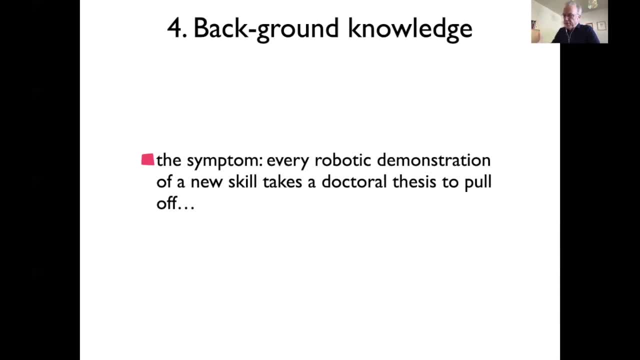 there are special purpose tasks always, and there's a lot of work going into solving these tasks and they're still not very good at it, And so a large portion of that is that background knowledge And you could say when you build a skill. 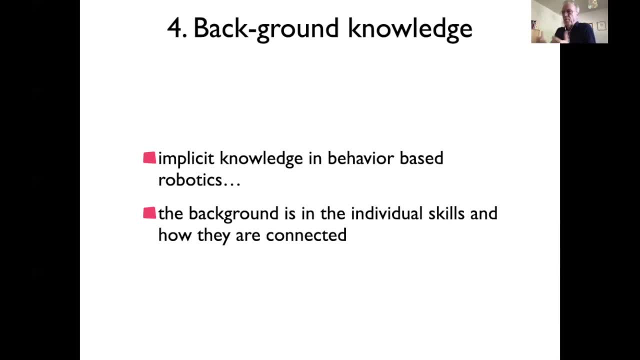 you enable the robot to have a certain behavior, as in the behavior-based approach, where they build different behaviors. That is sort of background knowledge, because you could say, in these skills is knowledge. I mean when you learn how to ride a bike. 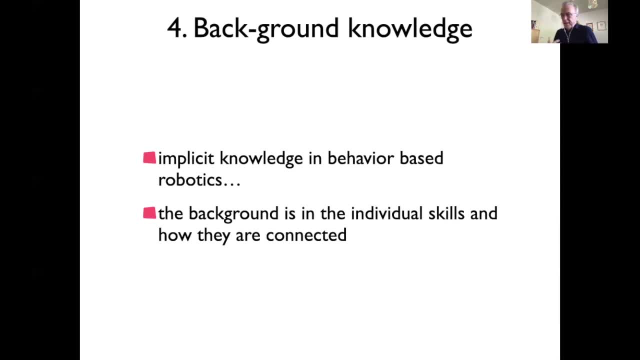 then you have acquired world knowledge about how bikes work, And that takes a lot of time. Or if you learn how to use a typewriter, or if you know how to communicate with others, you have skill and that builds world knowledge. So that's one approach of how to solve that. 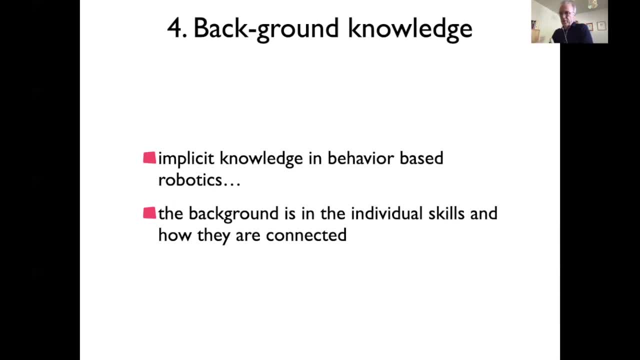 and would be a question of having a theory of tasks. What are the sort of skills you want to do? So one approach, One of them, is reinforcement learning, machine learning. That's certainly the hope that you could build skills that way. It has a terrible problem of the size of the workspaces. 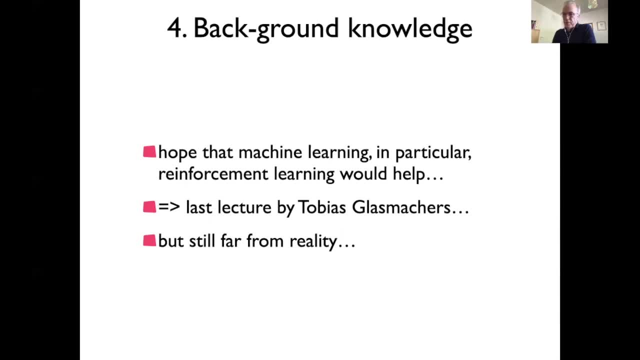 and the need for the difficulty of generalizing. There's a lot of work into that, using notions of having some primitives or some building modules and so on. So the last lecture in this course by Tobias Lausmachers will be reviewing reinforcement learning and you will see, I think, from that.